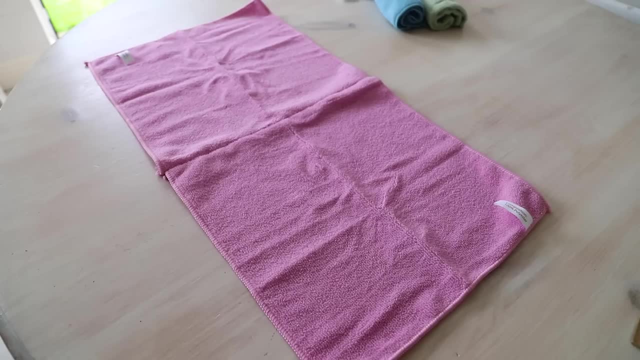 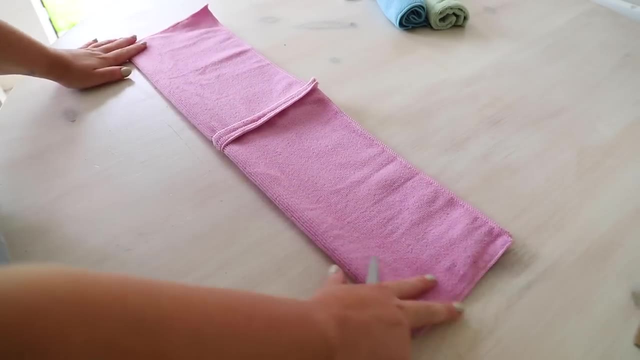 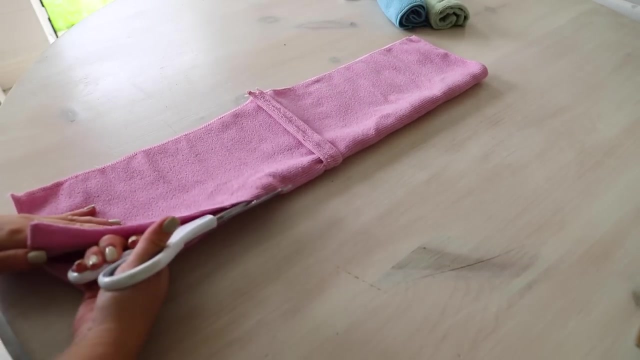 Do a straight stitch down one edge, and then I now have a long piece of microfiber fabric that I am then going to fold in half and cut it. So now I have two long strips. They measure roughly 25 inches is the width and the length is roughly 24-23.5 inches. Don't worry too much about the length. 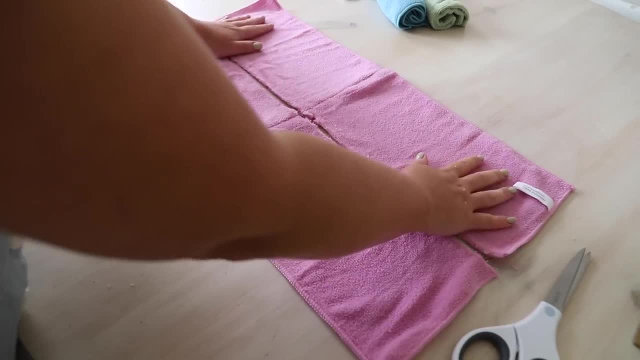 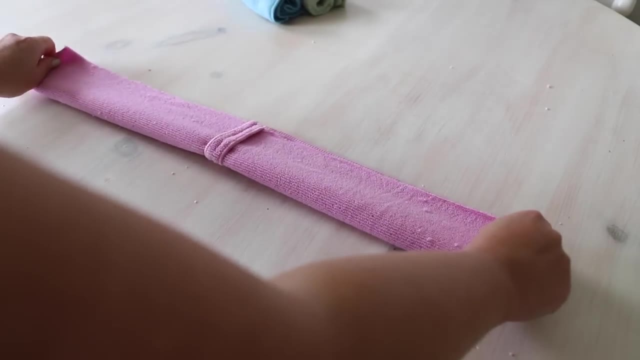 The longer it is, the more chunky it is going to be, and the shorter it is, the less kind of ruffles you are going to have. The length is anywhere from 22-25 inches. Let's work on one scrunchie at a time. So take one piece of fabric, fold it in half. 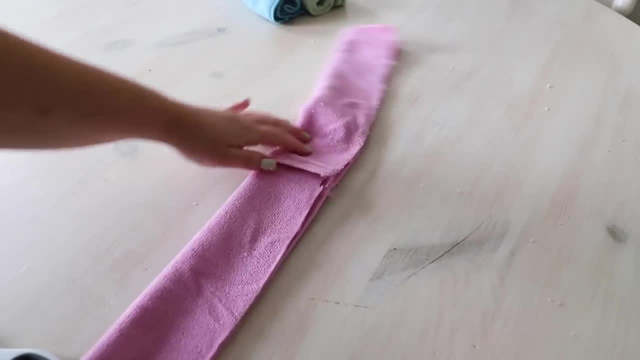 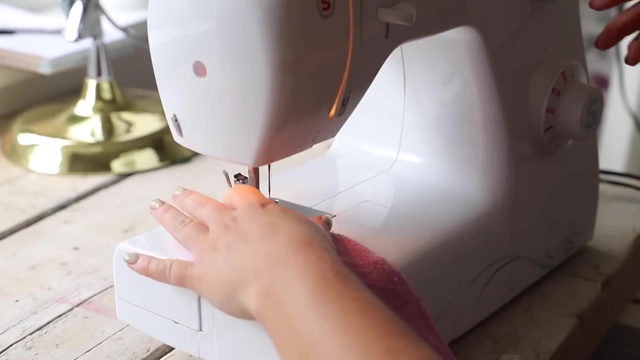 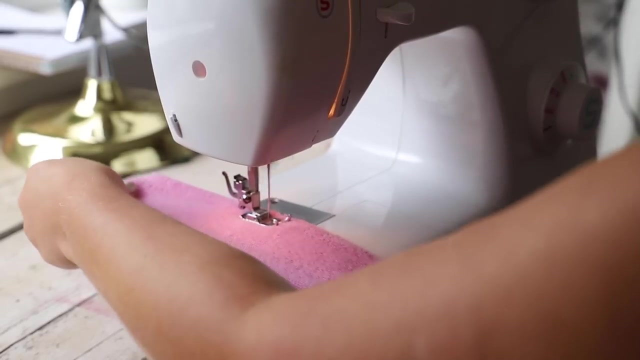 and straight. stitch down that lovely long edge. Do a reverse stitch at the beginning and the end so your stitch doesn't unravel. Pull it through and you are going to be left with this lovely long tunnel. Also, there is a burrito method of making towel scrunchies, which I did see online. 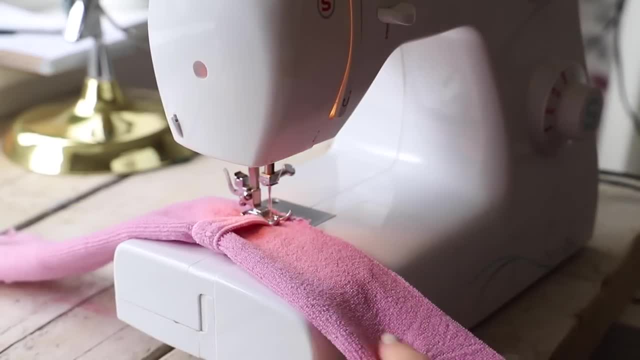 But I just found out that there is a burrito method of making towel scrunchies. But I just found out that there is a burrito method of making towel scrunchies. But I just found out that there is a burrito method of making towel scrunchies. 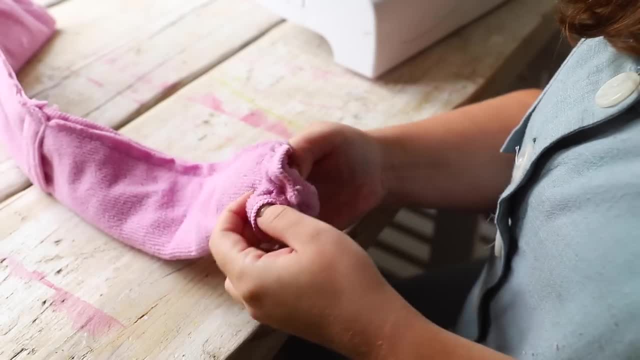 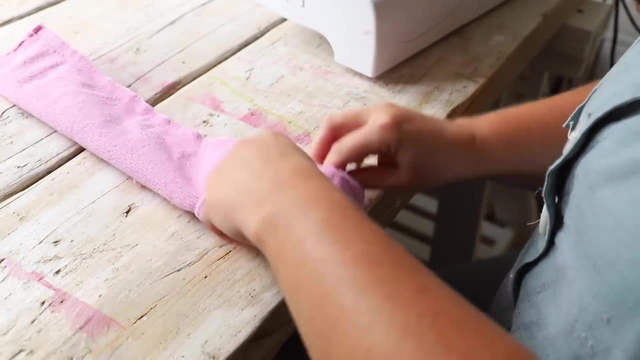 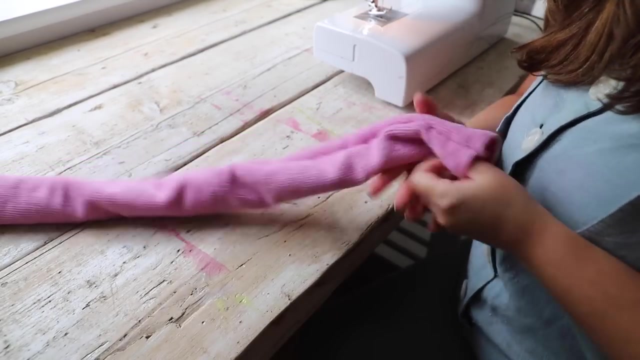 You could also make these with towel material, But from having a little look online, a lot of people prefer the microfibre cloth because the micro fibre cloths are super absorbent and when it comes to moisture I also seen a girl using the touches generate too much moisture, as she putting the scrunchies to puff up a bun in her hair. 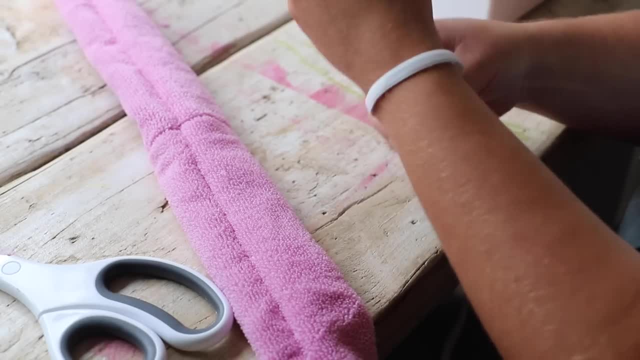 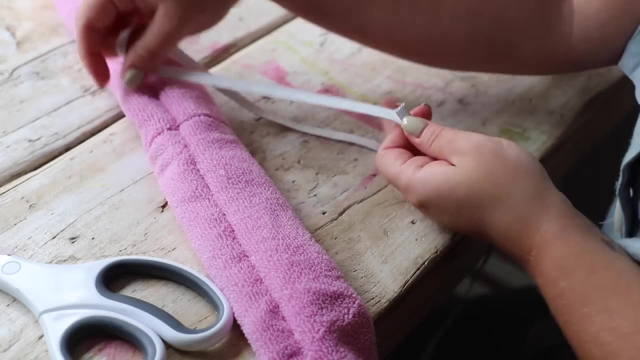 because the scrunchies were going to absorb some of the moisture excess water. so there's a few little things I learned from looking online. so now grab a piece of elastic and I like to roughly measure it. when you are making something custom, you may as well. 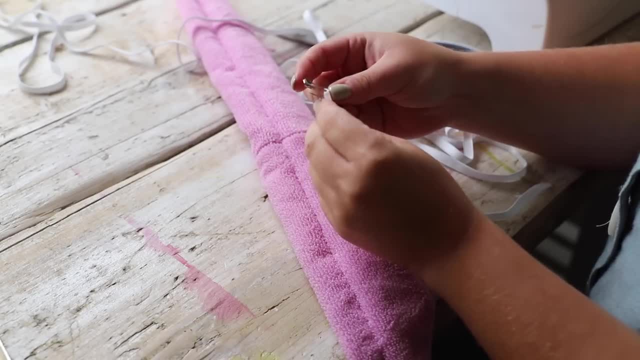 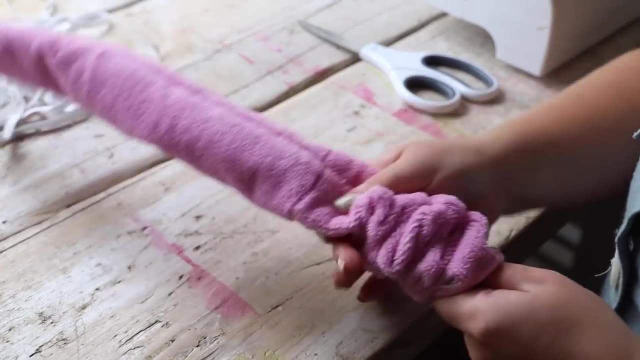 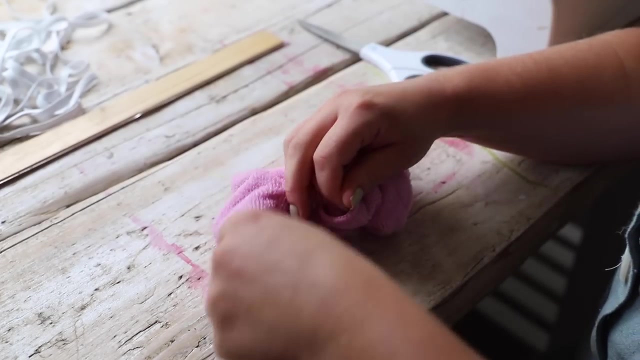 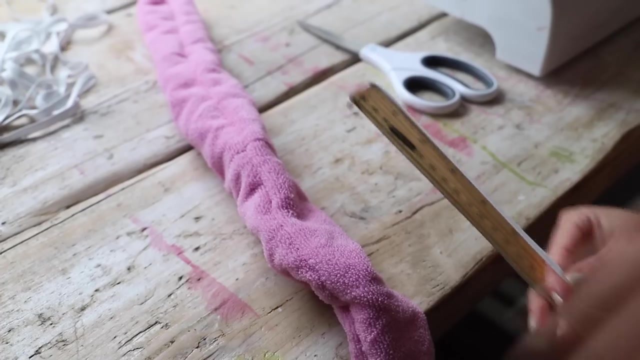 make it to fit your wrist, and I have quite a small wrist, so I'm popping the elastic around my wrist and just adding a little extra, giving it a snip. the extra that I'm adding on is just for when I tie a knot, when I slide it through the tunnel. I just don't let the elastic go. I found it tricky. 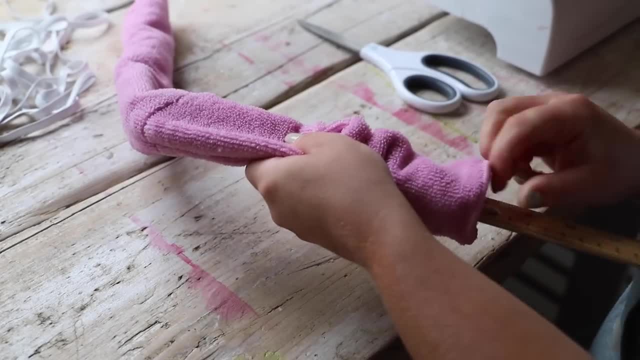 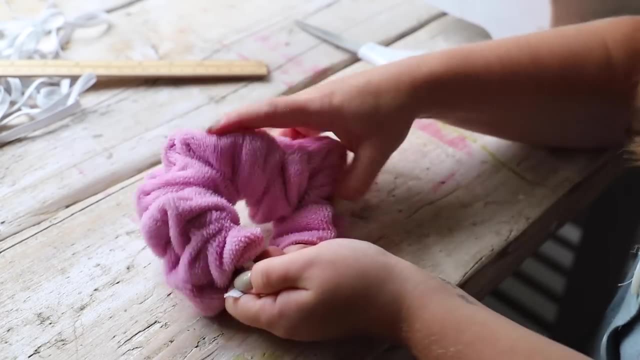 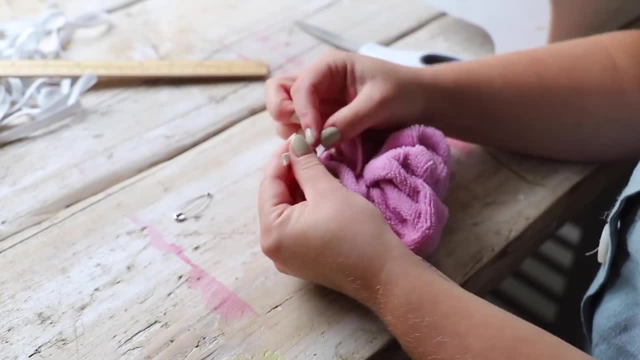 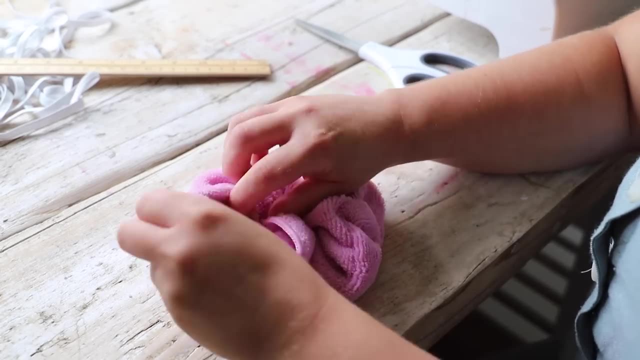 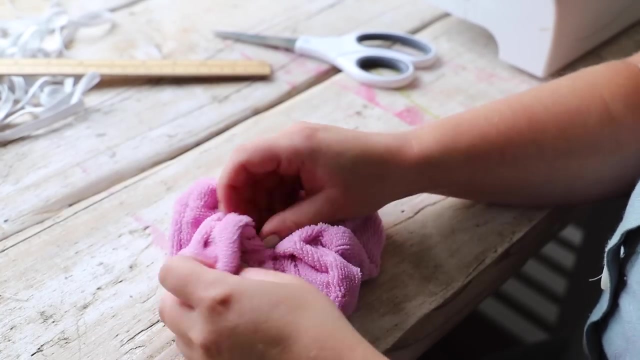 easier ways to do this, but that's all I had to hand. so now we're going to close up our scrunchie and we are done. so you're going to want to get that opening closed. so I fold the raw edges in on each other and I slide one on top of the other, so I'm basically sliding the tunnel in. 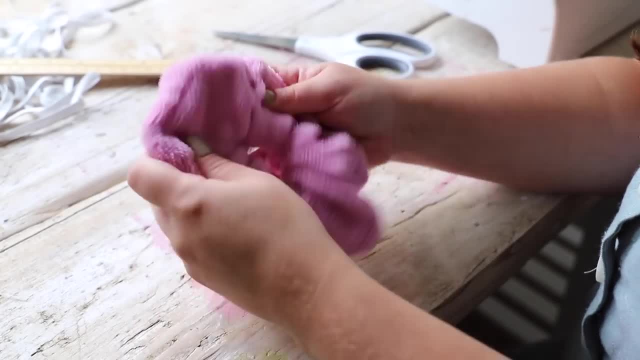 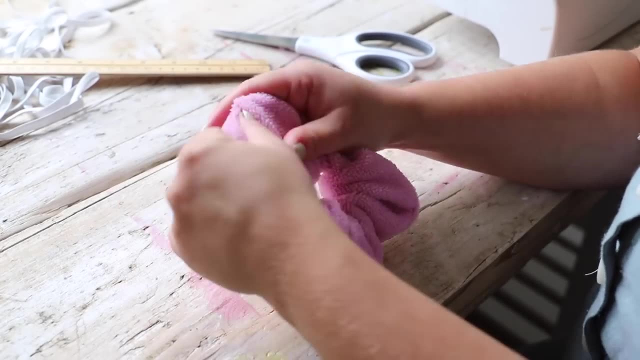 on itself, if that makes any sense. and then you have two ways of closing this. you can hand stitch it, which will be the more professional option. you could do a ladder stitch all the way around, or I'm going to take it to the machine and I'm just going to do a simple straight stitch. 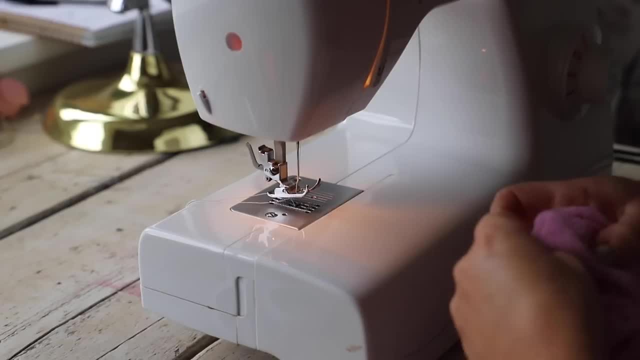 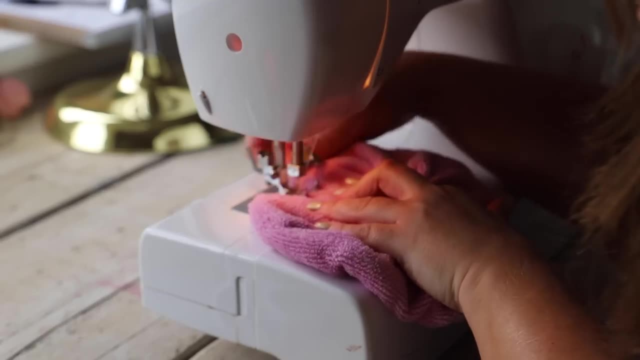 across that opening to close it. if you're doing a batch of these, that's going to be the quickest way to do it, but it mightn't be the prettiest. however, I find with a microfiber cloth you don't really notice the stitch and you get away with it. 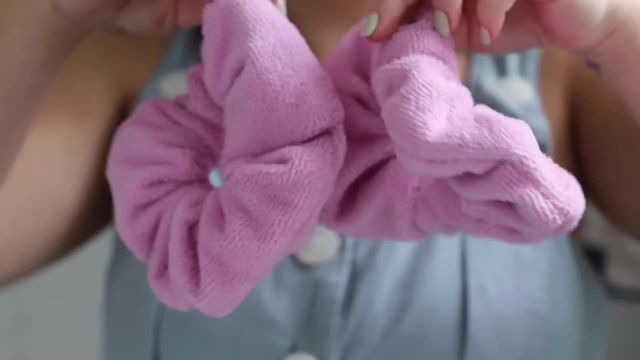 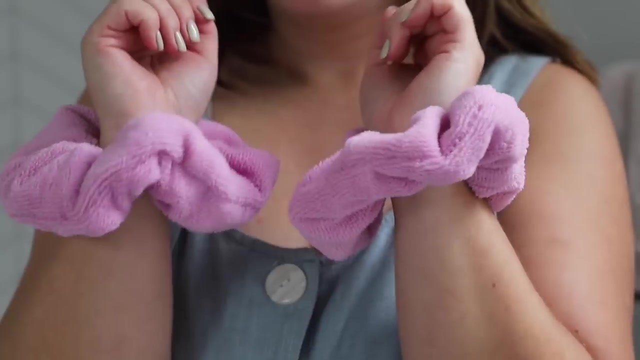 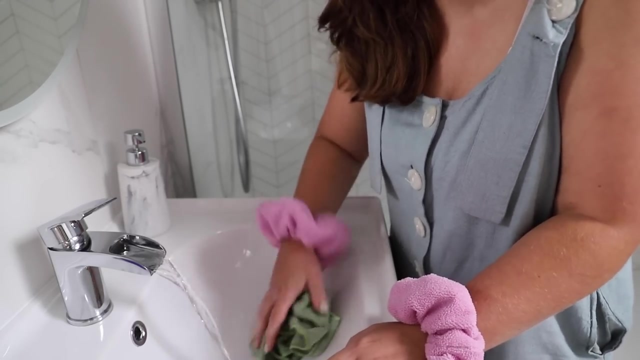 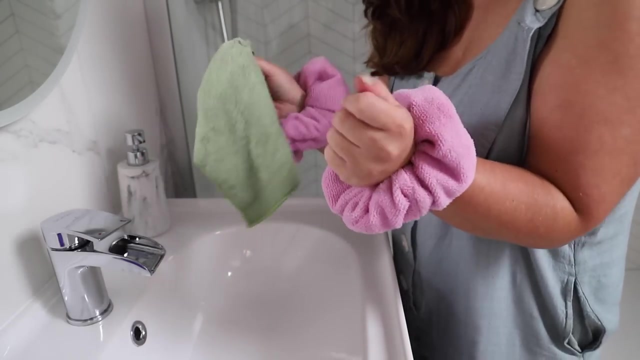 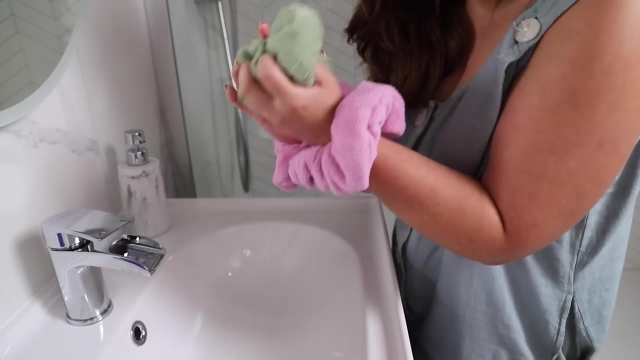 so okay, so I'm going to go ahead and do that, and I'm going to go ahead and do that and I'm going to put these to the test. so the idea is: okay. I know you wouldn't use this much water for washing your face, so the idea is: we don't want drips dripping down the arms, so washing my face, yeah, it's working. 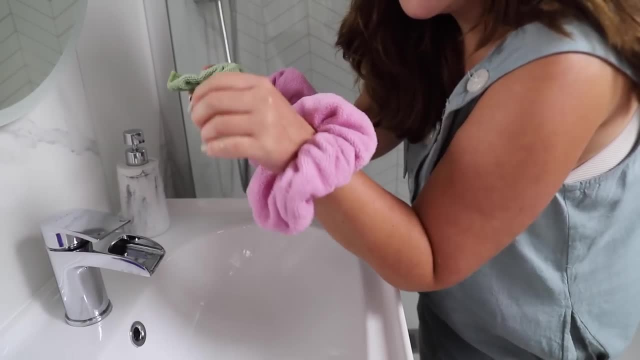 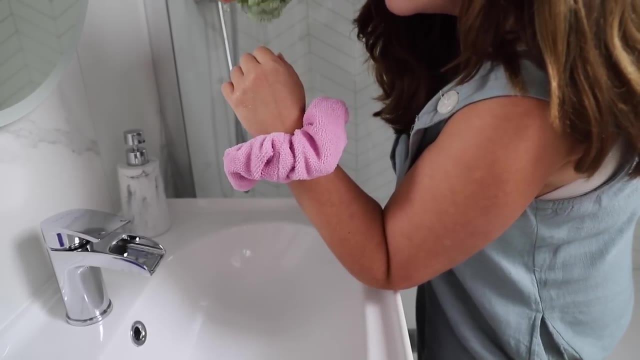 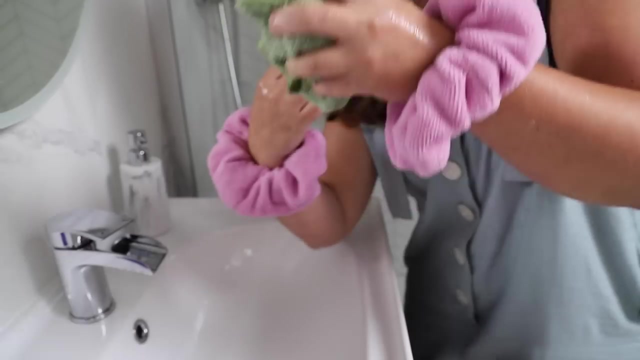 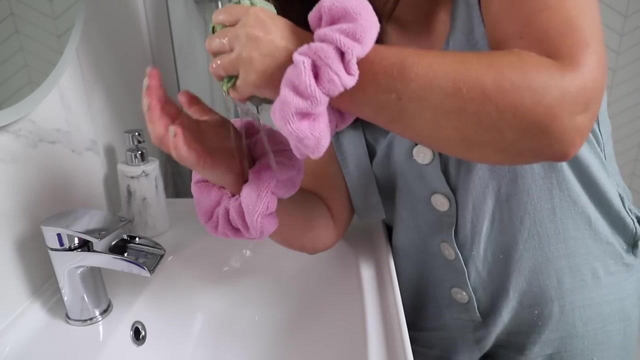 hang on if I go like this, because that would be the angle. oh, it is working. look, we've no drippy coming through at clinical trials. oh yes, tiny little dribble coming out there, but not as much as if I just went dunk. okay, let's try this one. yes, it's stopping. it is working, I can confirm. 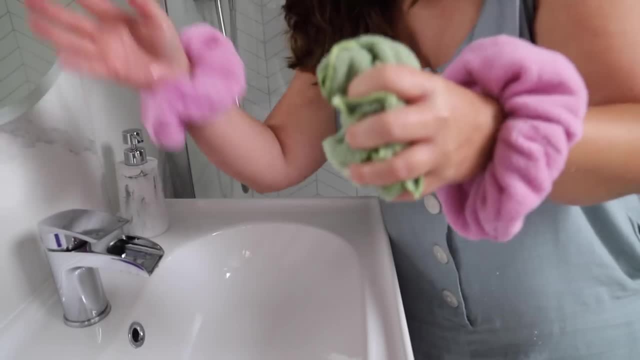 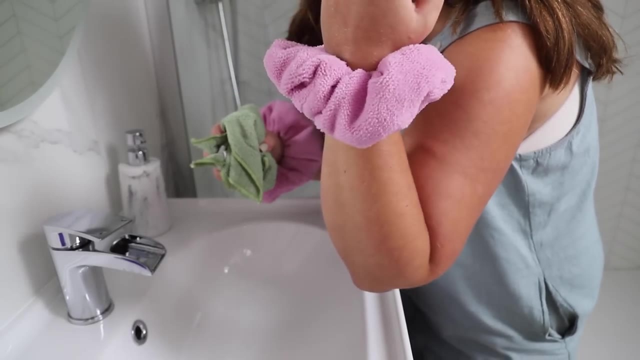 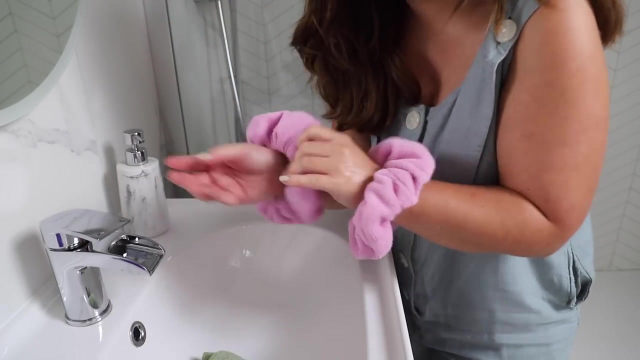 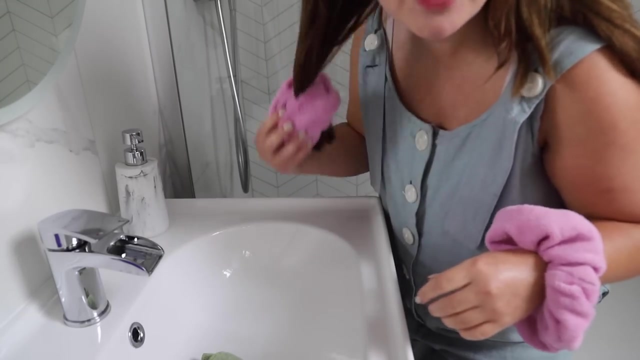 yeah, I don't look. there's no drips- no drips. also. apologies for that. I don't look. there's no drips- no drips. also apologies for that noise. in the background there's builders outside. these are success. and also they do work in your hair: shaboom shabam. they're quite chunky in your hair, but 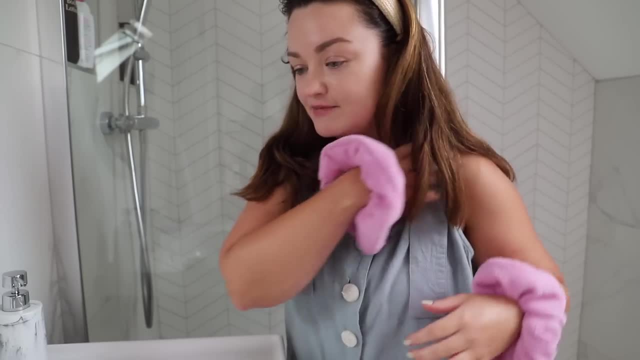 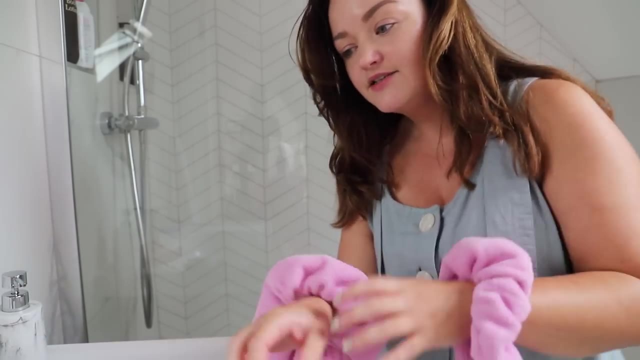 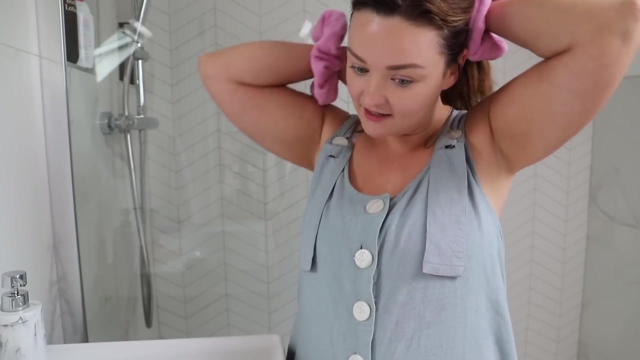 apparently hang on. I've only BB cream on my face because I wasn't planning on shooting my face today. I was just sewing and I have heard people using these to absorb excess moisture in the hair, in your hair. so let's say you wash your hair and you've tell: dried it, and maybe I don't know you're doing your. 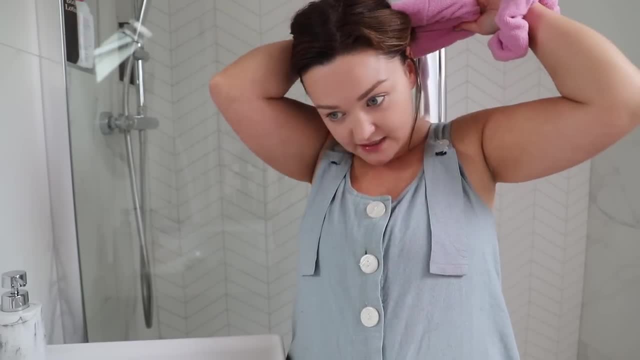 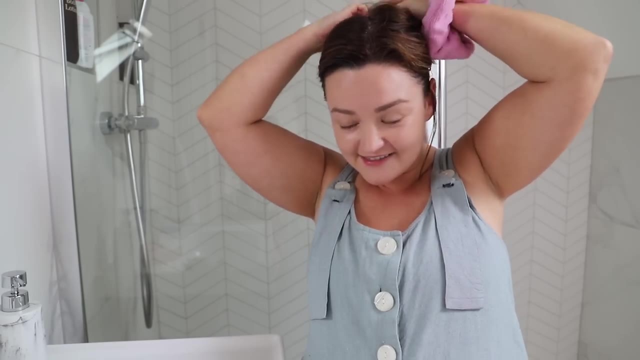 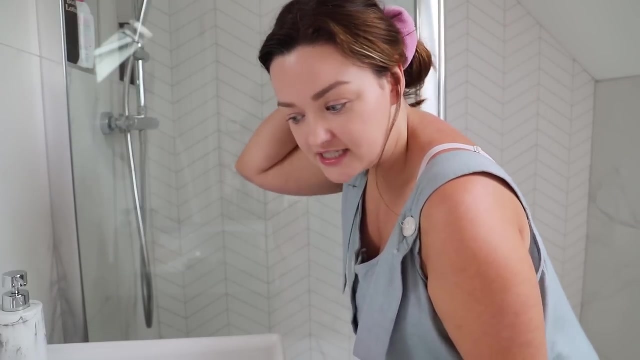 makeup or you're doing something. this girl put her scrunchie in her wet hair, in a bone, like kind of like this, kind of like that, and she was saying that the microfiber scrunchies absorbed more of the water while she was doing her makeup and getting ready. so 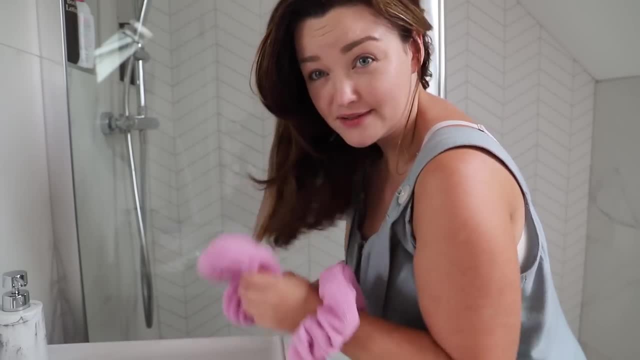 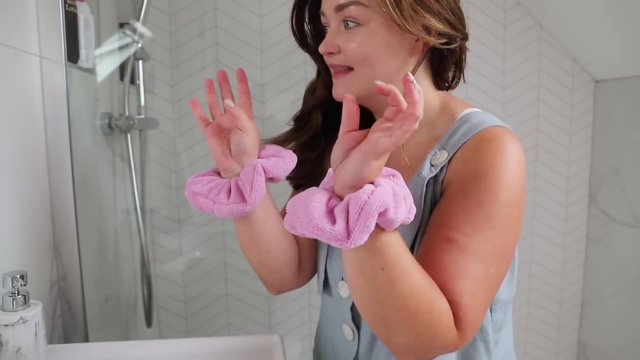 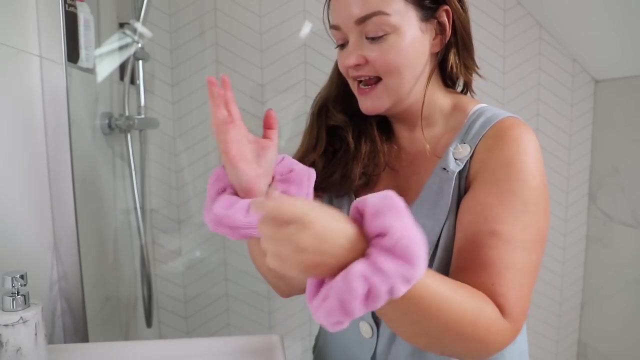 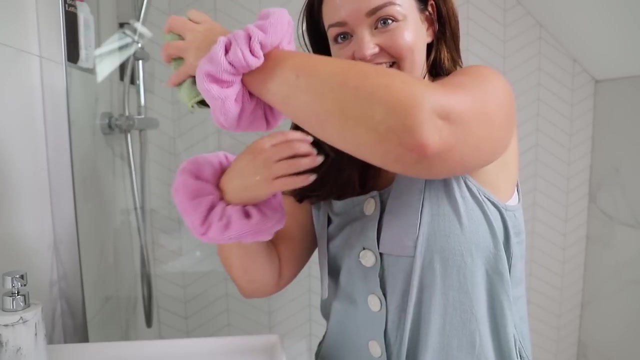 just another little thing. I learned about microfiber scrunchies but the goal of mine was to make them for my pal Karen, who had seen people and wearing these deal in their skincare and stopped the washer dribbling down their hands, and I can confirm that they do the trick. let me know if you make them. they're quite fun. okay, on to the next project. 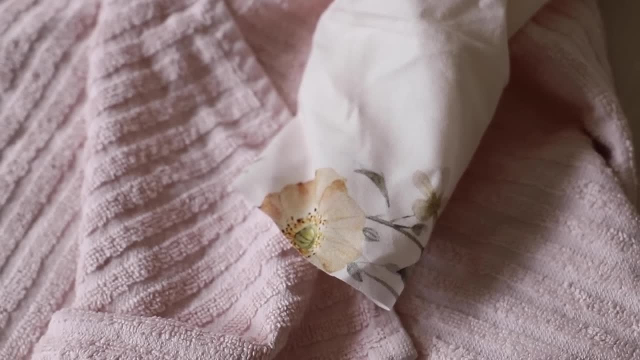 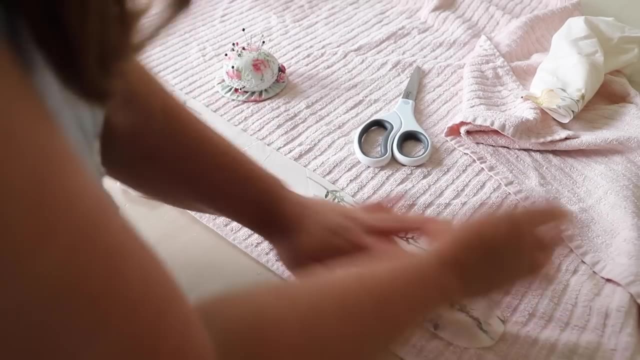 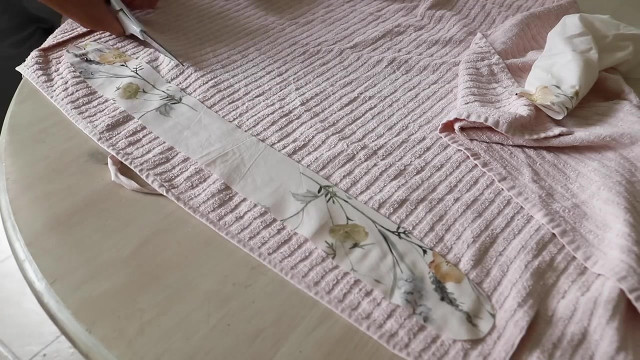 grab an old towel and some scrap fabric and we're going to make a really pretty headband that you can use for doing your makeup, doing your skincare. the idea of this one is to hold your hair back while you're doing your beauty bits. so you can create a template, a paper one, if you're making. 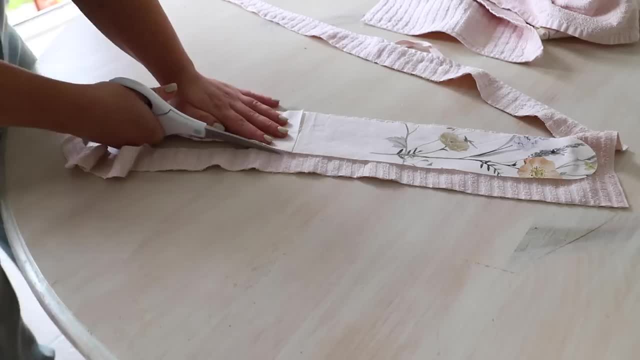 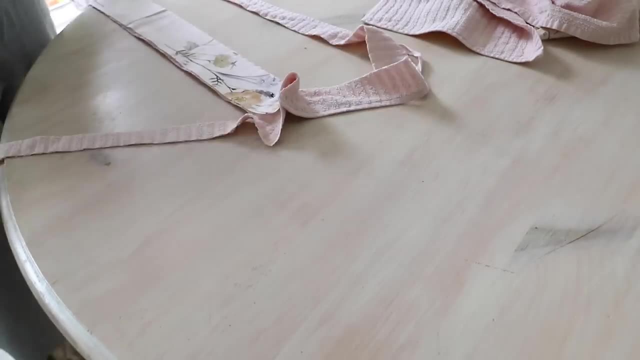 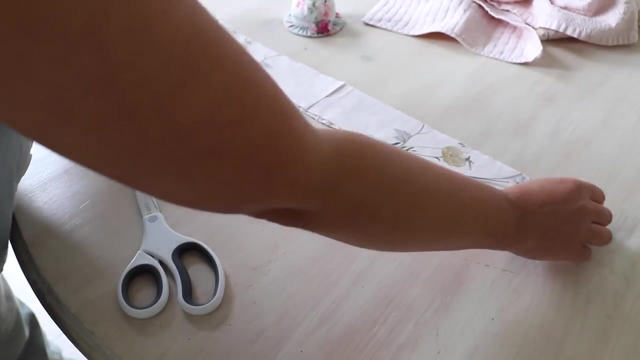 a batch of these, so it's going to be 25 inches in length, but you're going around the edges or you could do a different shape on the edges, you could square them off, but I just like the rounded edge and it's going to be 25 times 2.5, so 2.5 inches is going to be. 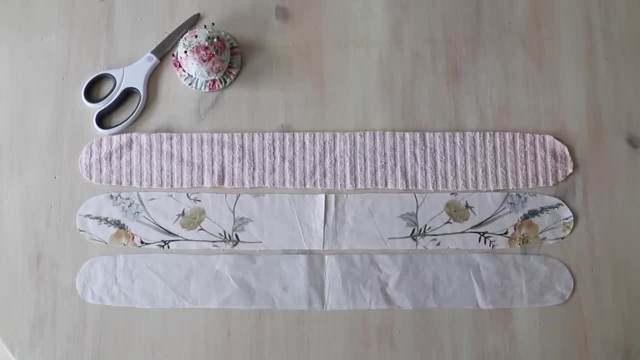 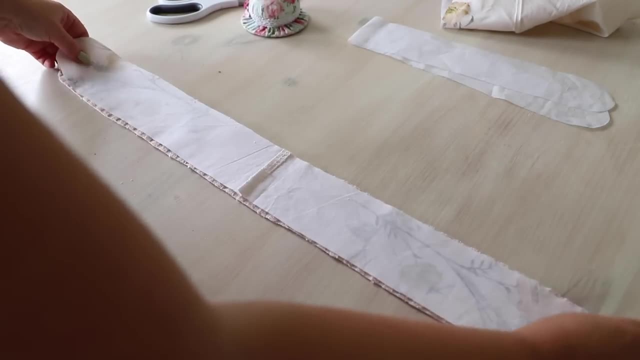 the width of your headband. you can make this bigger, you can make it smaller. I find for my size head, two and a half inches is grand. so place the two pieces of fabric together with the right sides facing each other. so that just means that the pattern and the pretty sides are. 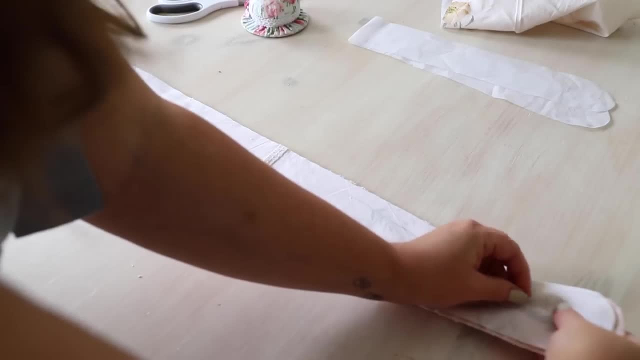 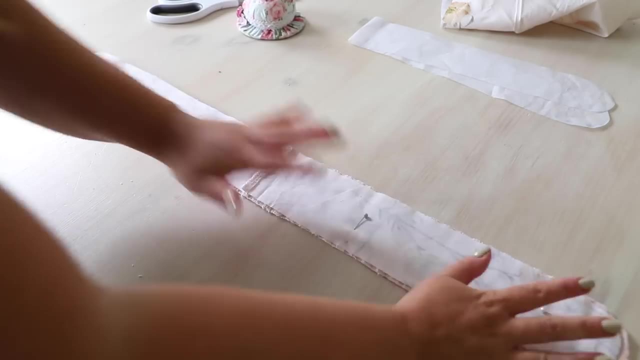 facing each other and then grab your sewing pins and pin the fabric in place. you're then going to stitch all the way around, but you are going to leave an opening so that you can pull it the right way through and make sure the opening is big enough that it's. 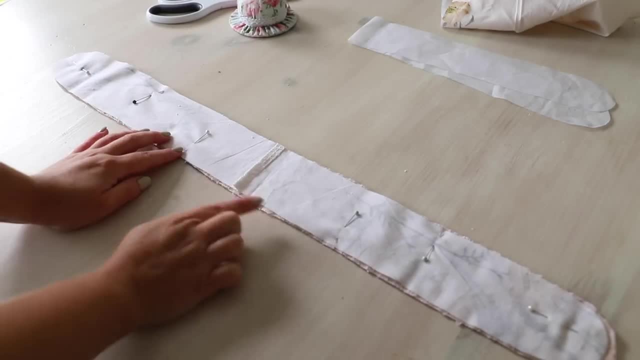 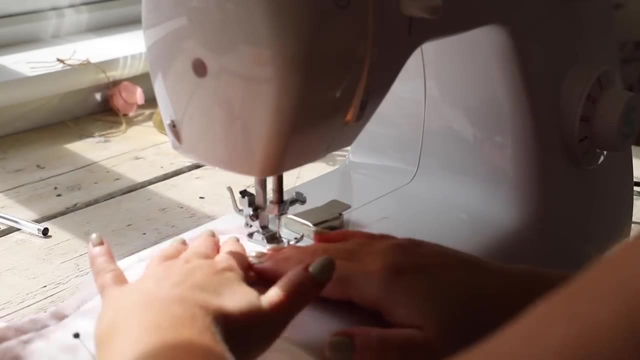 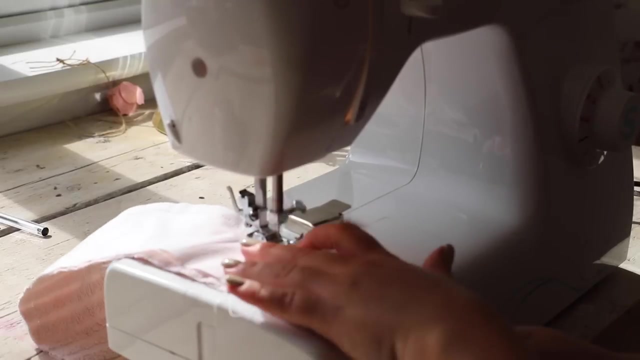 going to fit your hand. as I was making these, I was thinking that these would do really well in the likes of the wedding industry. so, for anyone who's new, I do have some cricket videos and I was thinking that you could possibly, if you were making these, to sell, if you. 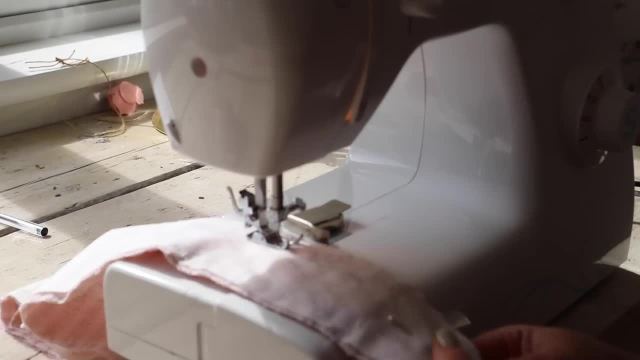 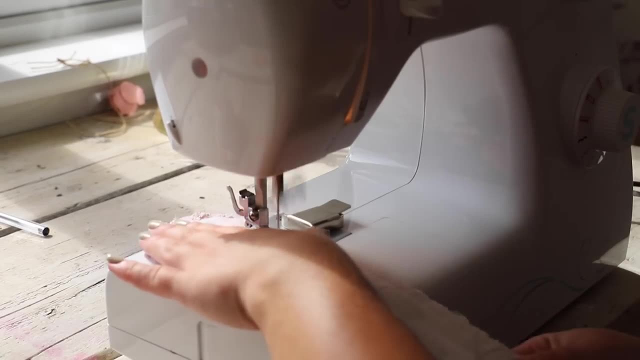 could personalize them with, you know, bride or bridesmaid and with some pretty fabric. I think if you were making these to sell, they would do really well if you could personalize them. so before turning them the right way out, you can trim off any bulk. so if there's any towel, 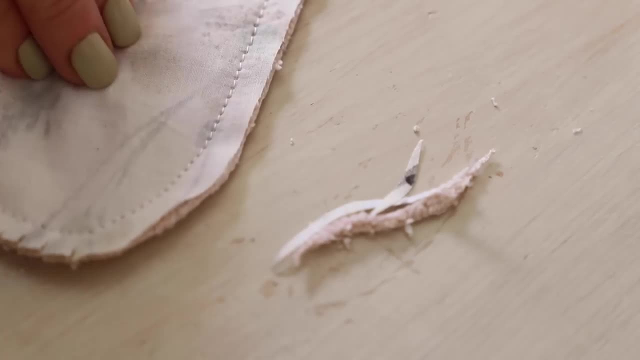 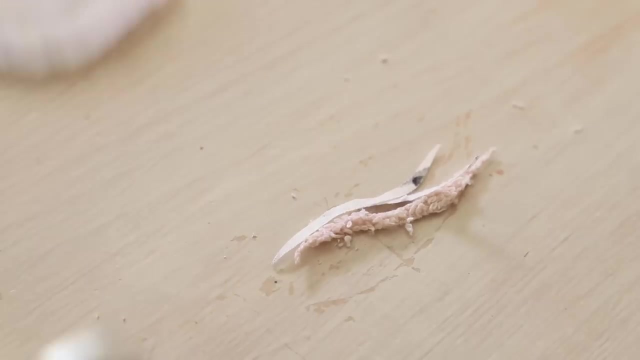 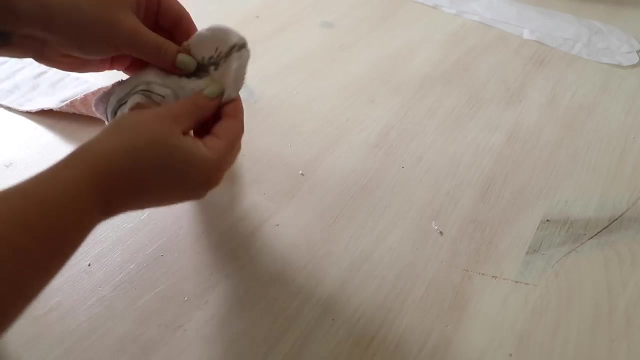 material that's a bit bulky and then you can just snip around the curves. this will just give you a better curved edge when you turn it the right way in. so get your iron handy and once you have it nice and fixed and it's the right way out, I like to give 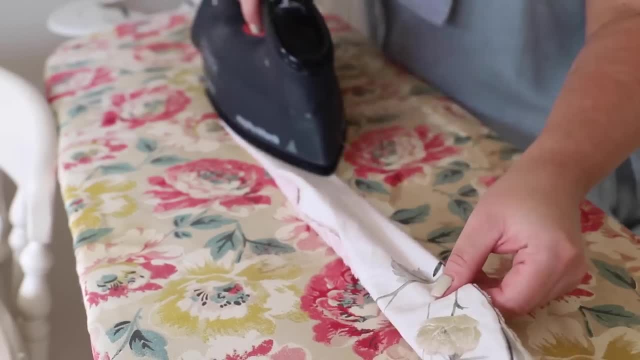 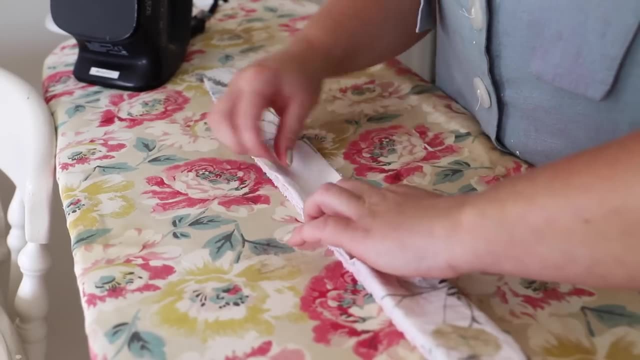 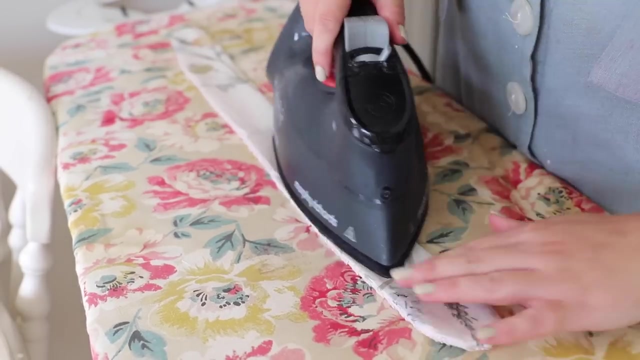 it a good press and iron that opening closed on itself before doing a top stitch to close everything off and give it a nice professional finish. so the iron is your friend here and that's going to get it nice and neat so you can take it to the machine and do a top stitch all the 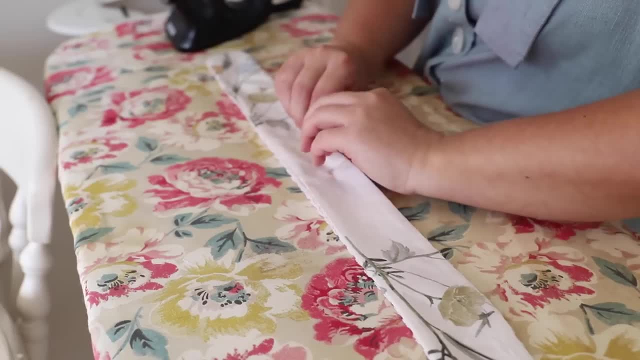 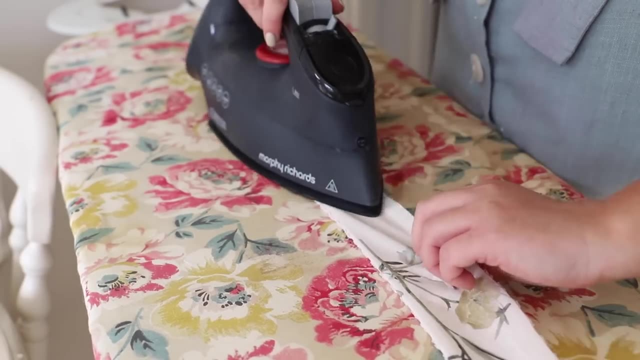 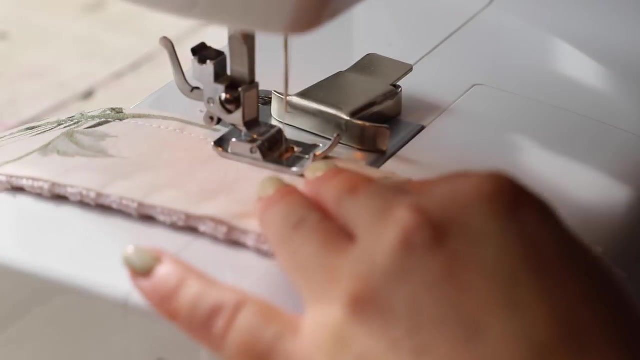 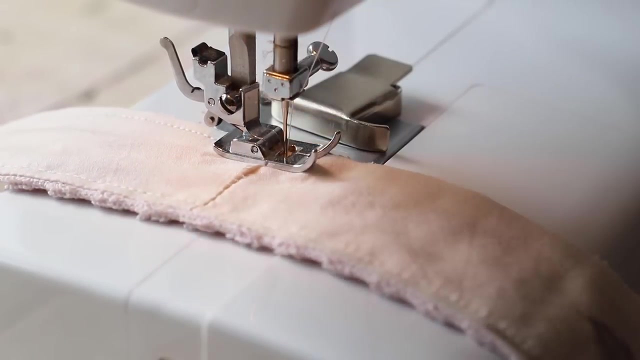 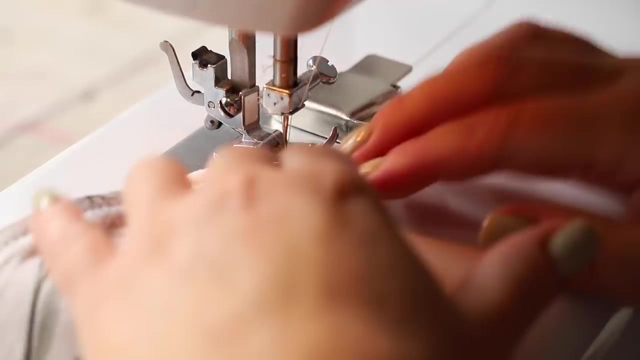 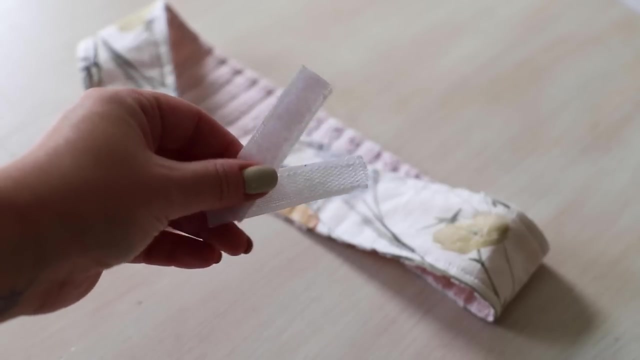 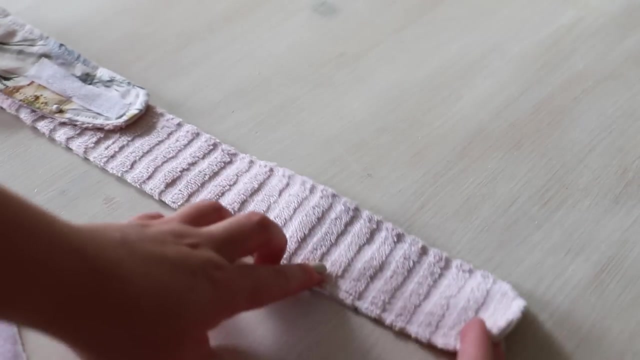 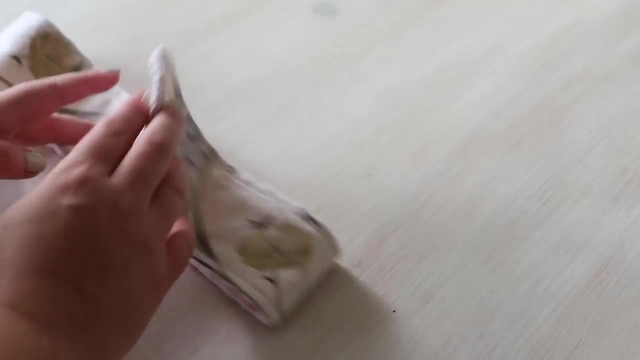 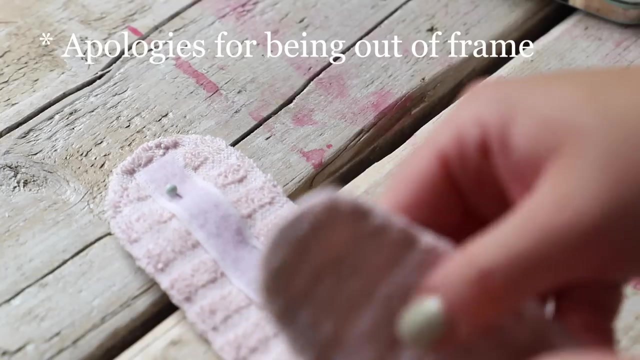 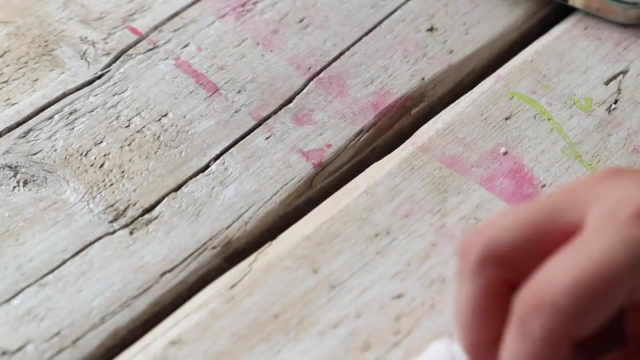 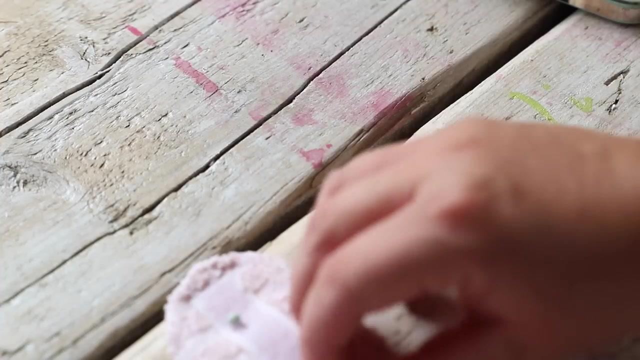 way around, and that will close your opening. and that's it for this video. I hope you enjoyed it and I'll see you in the next one. bye foreign. you will see it on this side, so I'm going to use some fabric glue to stick this on. not ideal, but I 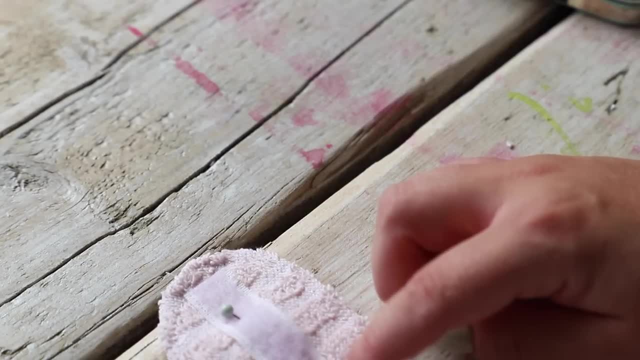 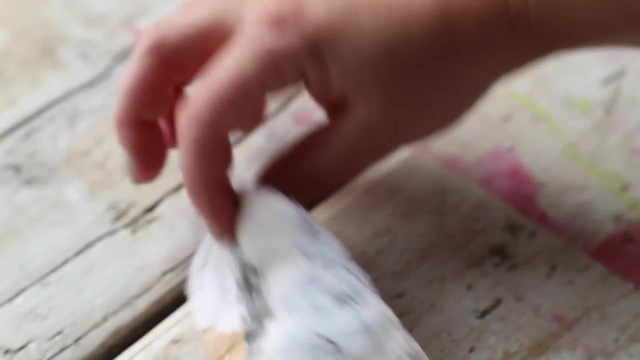 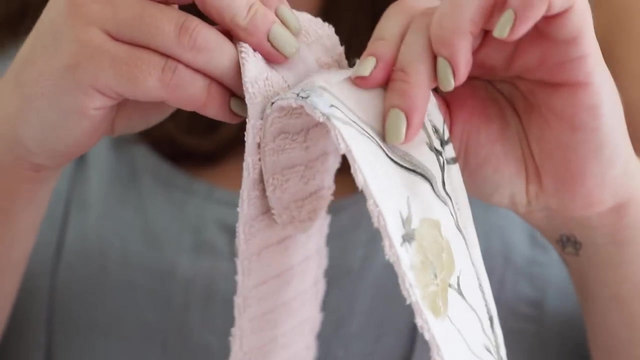 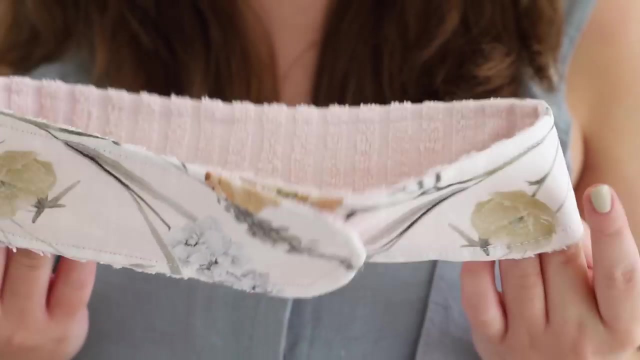 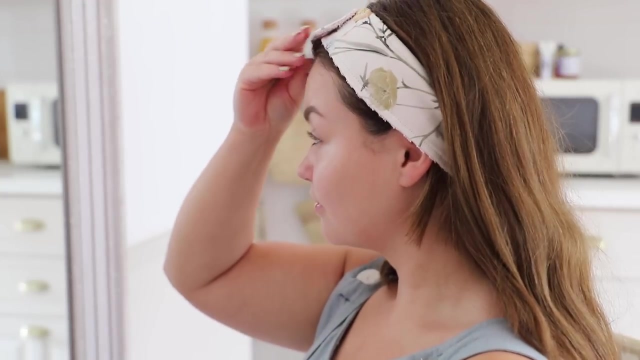 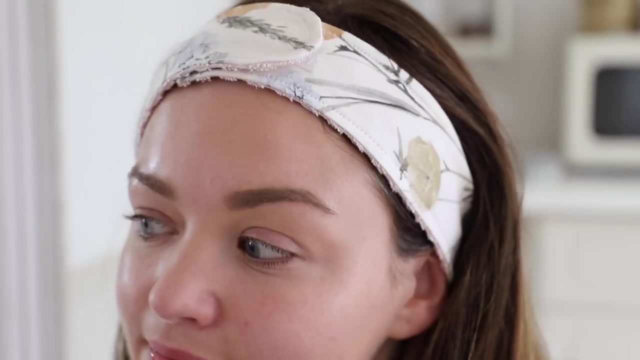 don't want to see a top stitch to avoid this. if you stitch this piece of Velcro onto this towel a couple of steps back before you sandwich the two of them together to stitch around, you can avoid that problem. J o e e, n o e e. 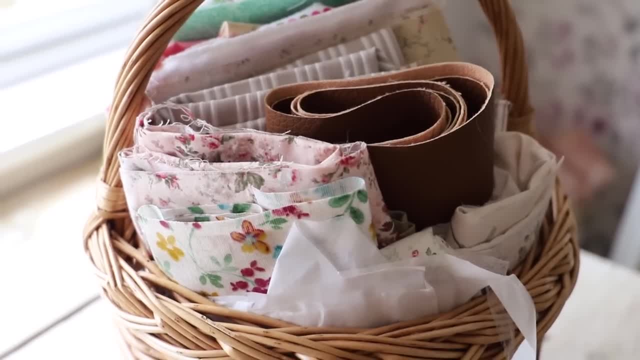 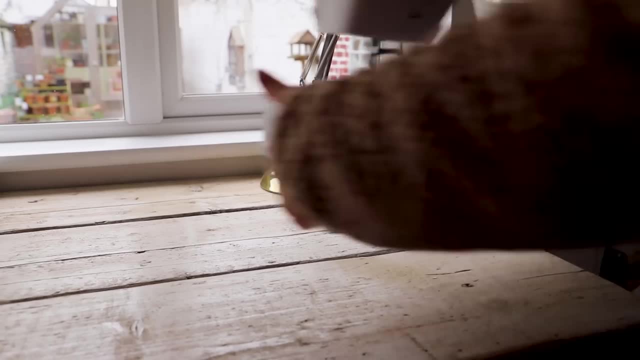 fabric and we're going to make some hand warmers. You're also going to need some treads, some pins, some rice and some essential oil, but that's optional. Give your fabric a good iron before cutting it, so there's no wrinkles in the fabric, and set up your machine. Put out two squares of. 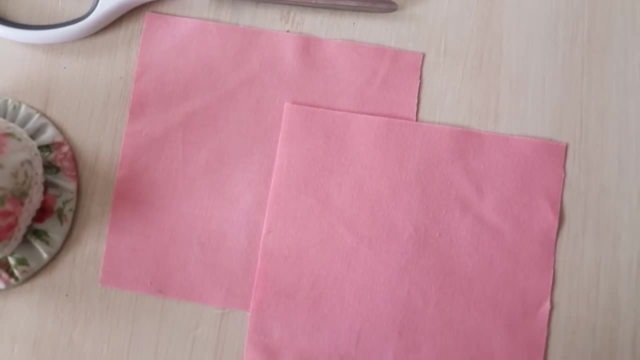 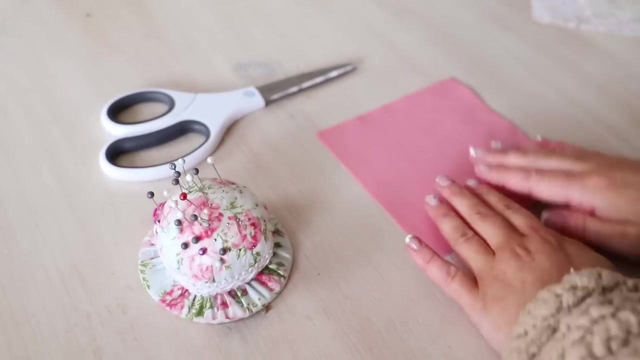 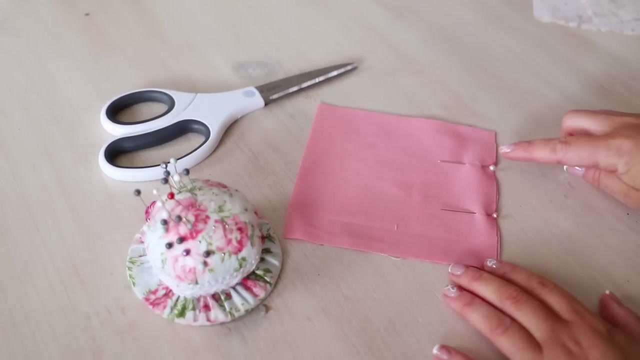 fabric that are five inches by five inches. Place the right side of the fabric together and line up the edge. Spin the fabric together and make sure to leave a gap large enough that you can turn it the right way out, and that'll also be big enough to fill with rice. Also, I used a half an inch seam. 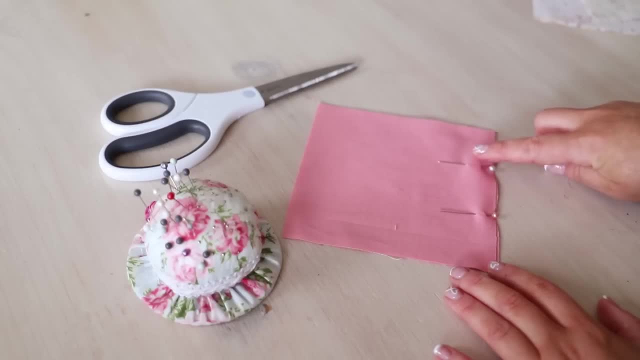 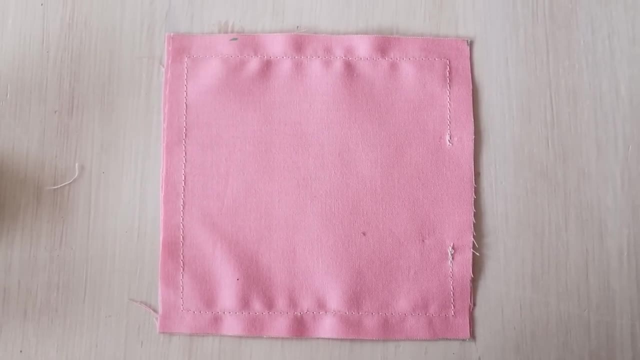 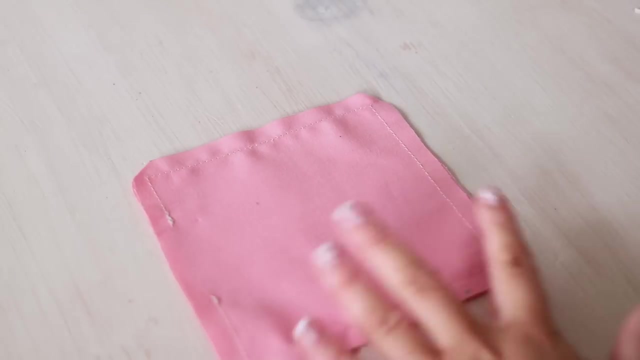 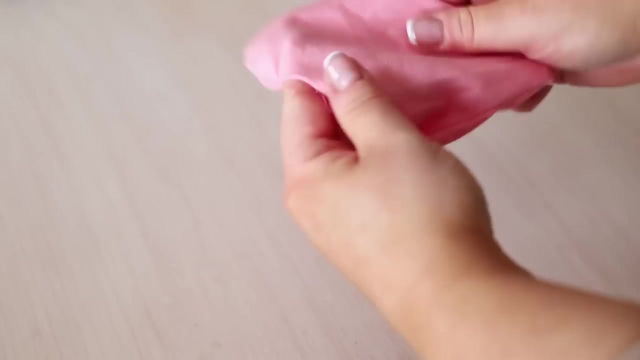 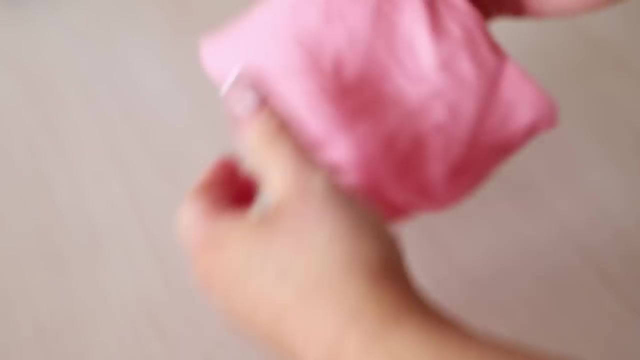 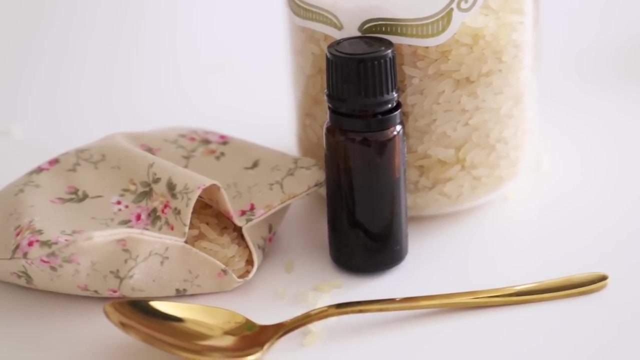 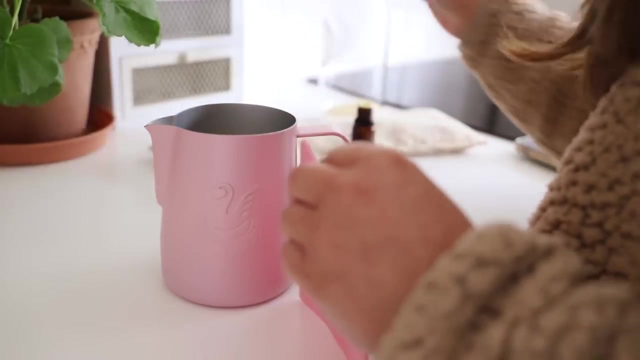 allowance for this. Before turning the fabric the right way out, I just clipped all of the four corners. You can use some paper as a funnel, if you need to, to insert the rice into the little bag that you've just made. but I had a jug that had a spout on it and I found that that was really. 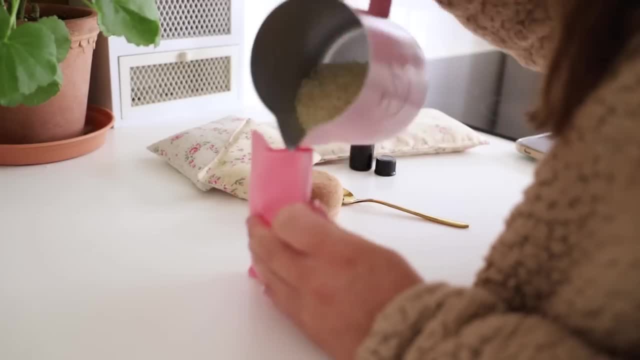 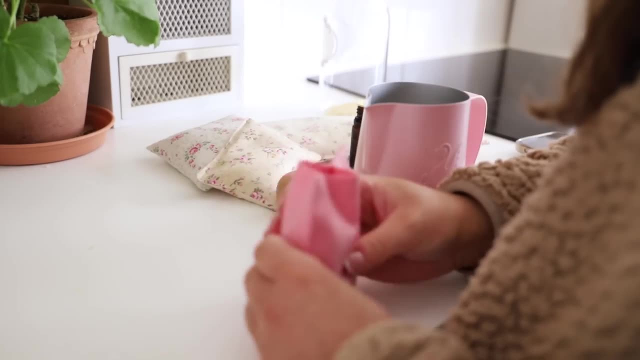 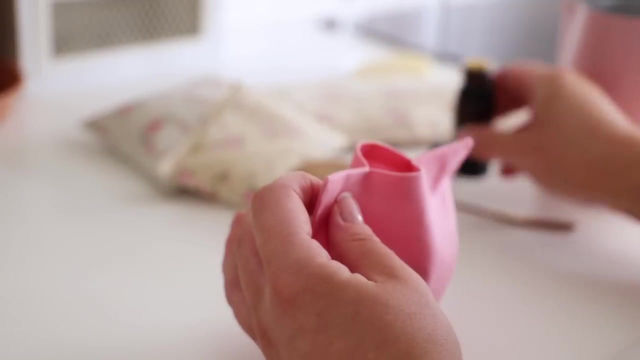 handy. I filled the bag about three quarters the way full and I left a gap so that I could easily stitch it closed. Now you could do a hand stitch on this, but would you believe me if I told you I had no hand stitching needles? They were too big. the ones that I had were too thick, so I just 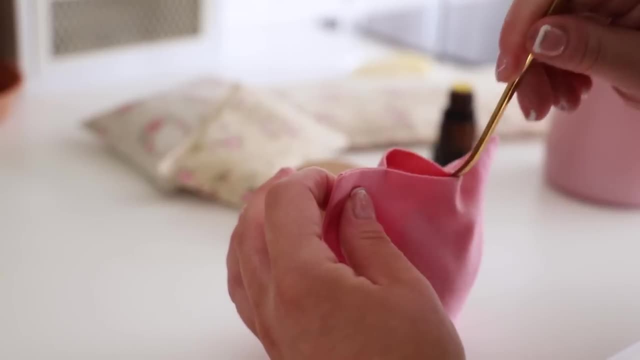 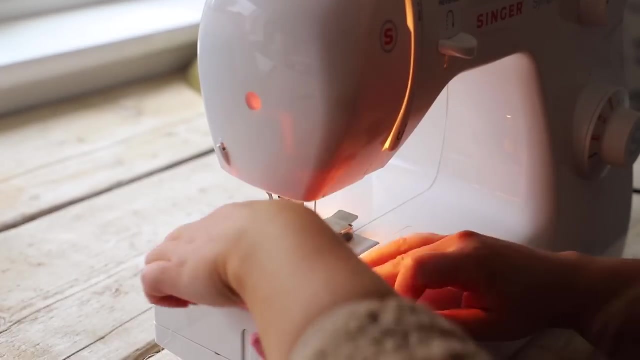 was lazy and I stitched a straight stitch across to close the gap. If you want to add some essential oils in- I added about three to four drops- You can mix the essential oil beforehand in a little bit of water and then you can add some essential oils in. I added about three to four. 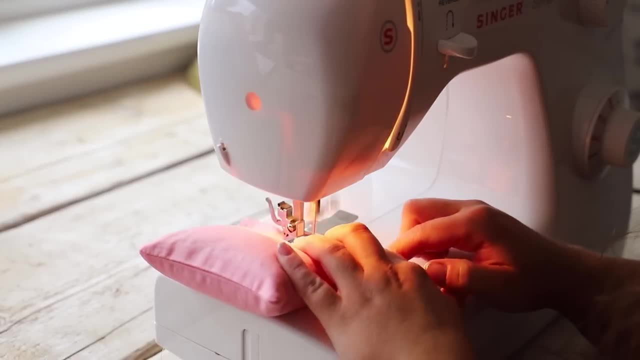 drops. You can mix the essential oil beforehand in a little bit of water and then you can add some essential oils in a little bowl. Just be careful when you're doing it, the way I am, that you don't get any essential oil on the fabric as it might mark it. To heat these warmers up, give them 30 to. 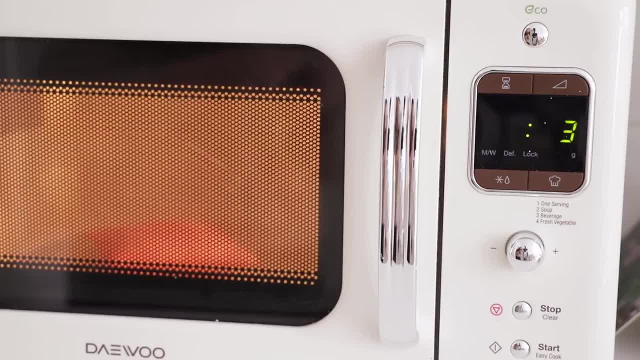 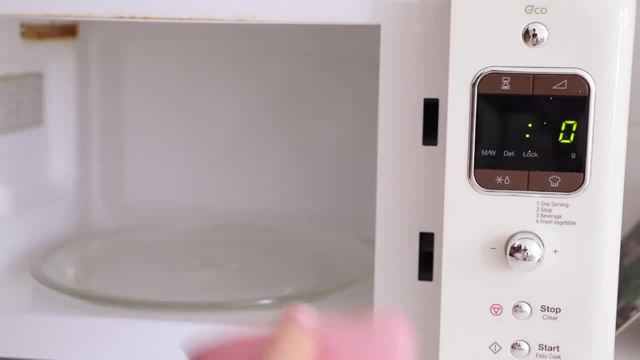 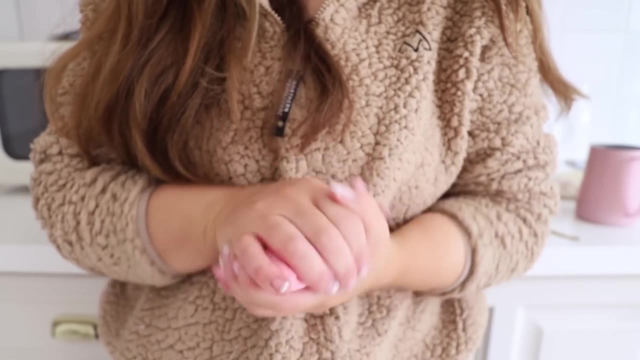 40 seconds in a microwave. I found 30 seconds was plenty, but it's going to depend on the wattage of your microwave. I also made a larger one that will be perfect as more of a heat patch so you could use on your shoulder or you could use it on a tummy when you have cramps. and this is 12 inches by 6. 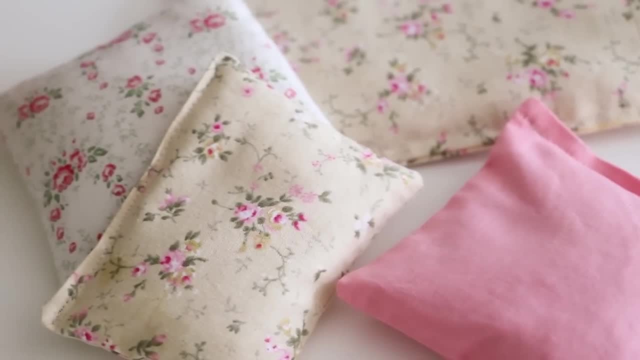 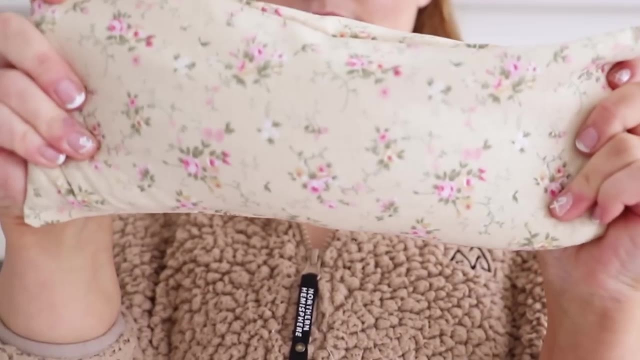 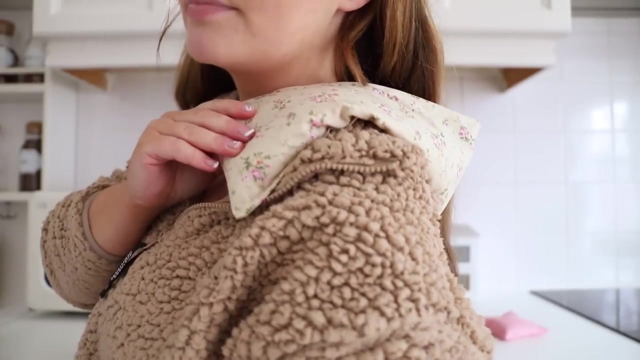 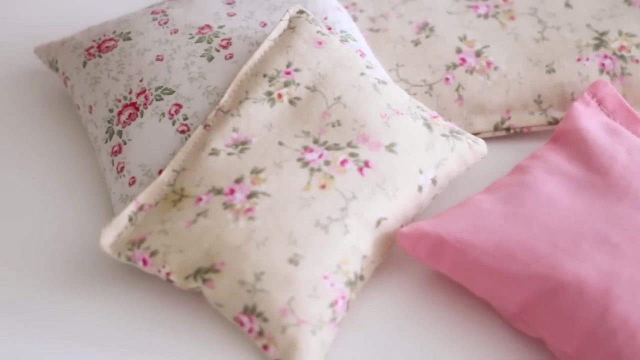 inches, If you want to try those dimensions for that size, and I found that that one took a bit longer to heat up. It took about a minute to heat up, but you could always start slow and then build up the heat. So if you've ever wondered how I get my hair curly without heat, well, a tiny bit of heat. 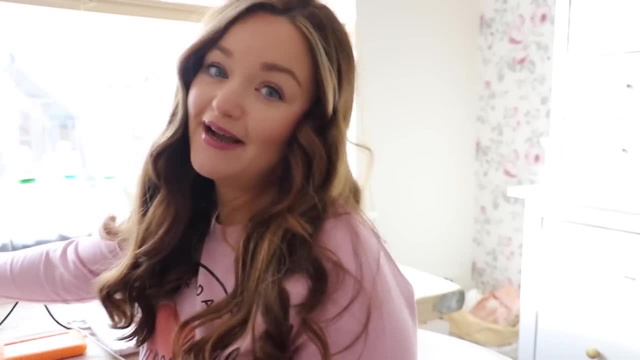 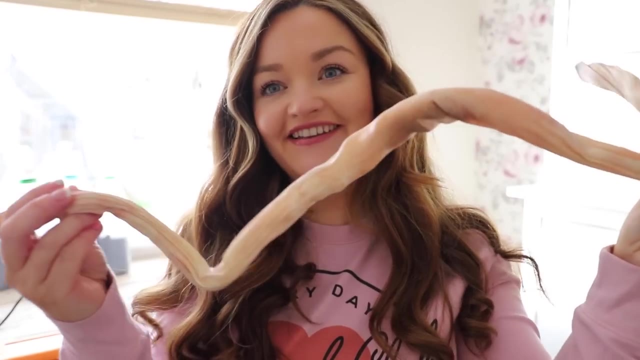 because you do have to dry your hair first. I use one of these but, as you can see, it's really bashed. So this is one. I bought its a heatless hair curler. Mine has been through the wars, As you can see. 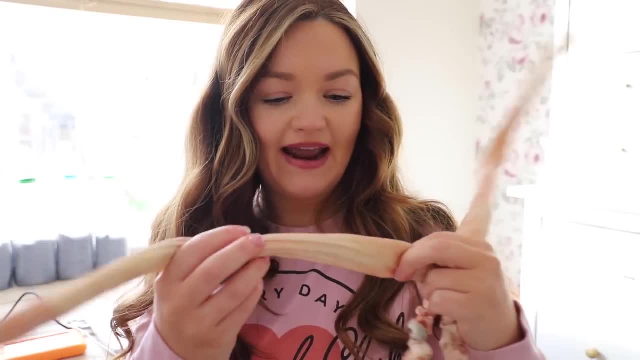 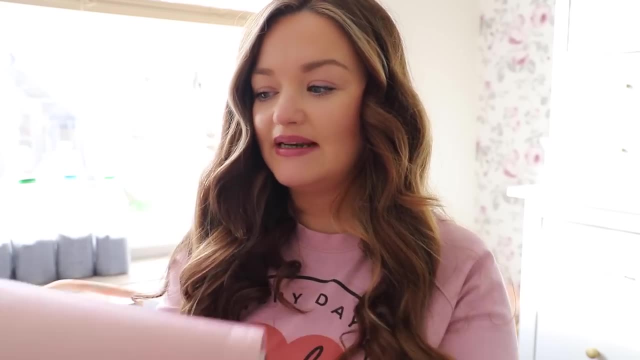 the sponge on the inside has just gone flat Hairspray on it. Yeah, it's not looking too fresh. I'm gonna make a new one. I have some like a satin kind of ribbon. I actually think this is Christmas tree ribbon. 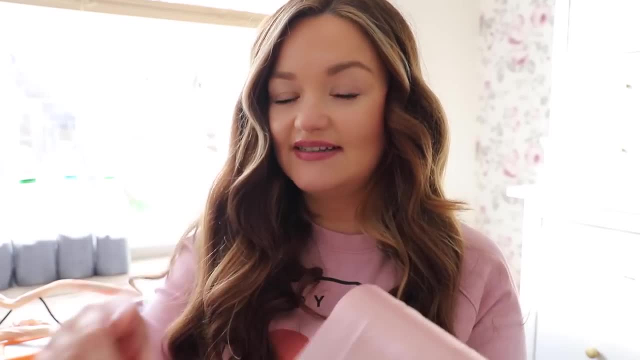 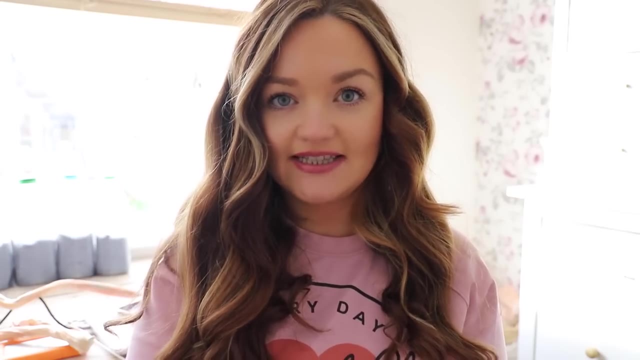 But This material is gonna be perfect to make a new hair wrap And I'm gonna show you how I make it and I'm gonna give you all the dimensions and everything so you can do it yourself. I'll give you a little demo at the end. 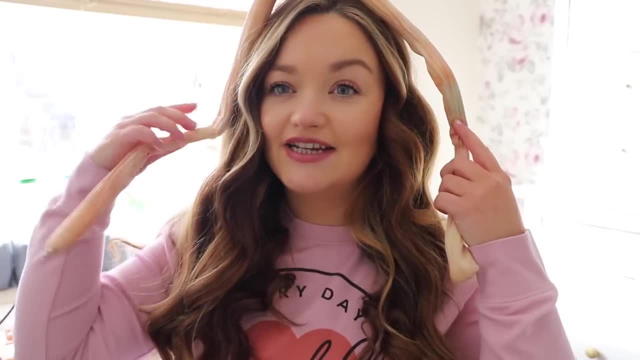 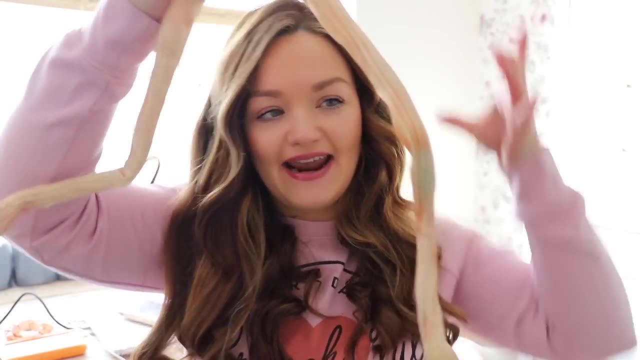 and I'll share how I wrap it around. I did actually the curls that are in my hair today I did actually do with my wonky one. If I had a nice consistent hair tube thingy, my curls would be a bit more consistent. 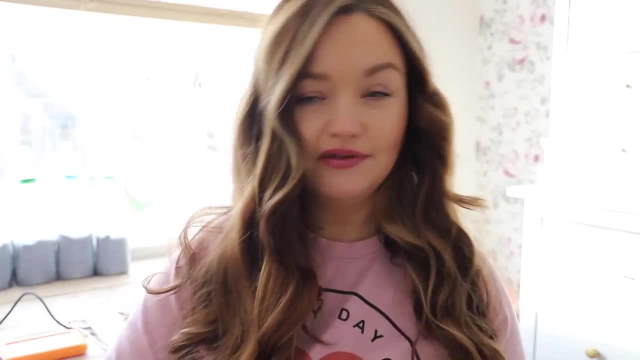 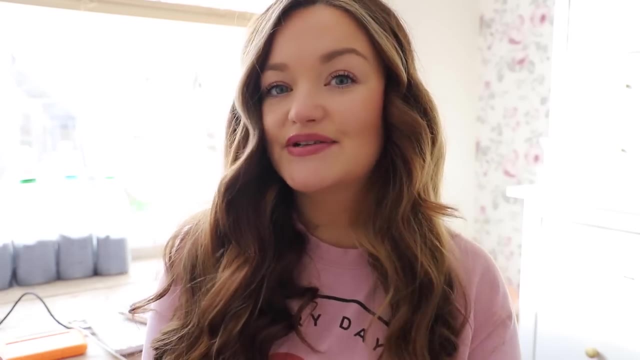 But anyway, this is what I do once you get this kind of tousled loose. look, I wash my hair in the evening. I just blast it rough dry with the hairdryer and then I stick in my curler, which I'm about to make a new one. 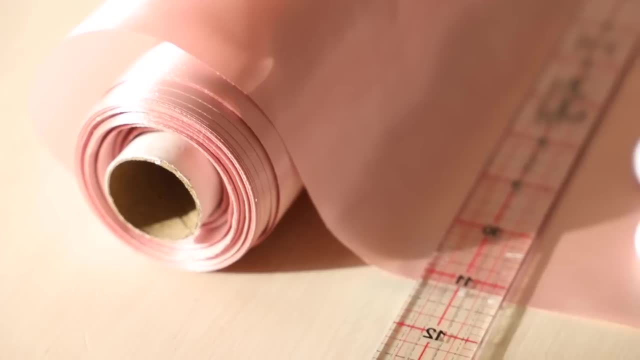 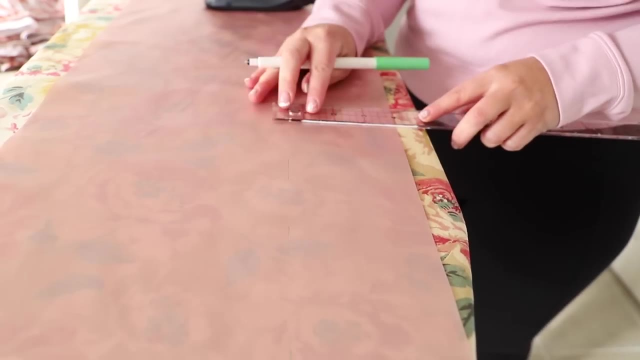 If you have some satin or silk fabric, that would be perfect for this project, as I read that it reduces the frizz in your hair. But do use whatever you have. So if cotton or poly cotton is all you have, you can still make this. 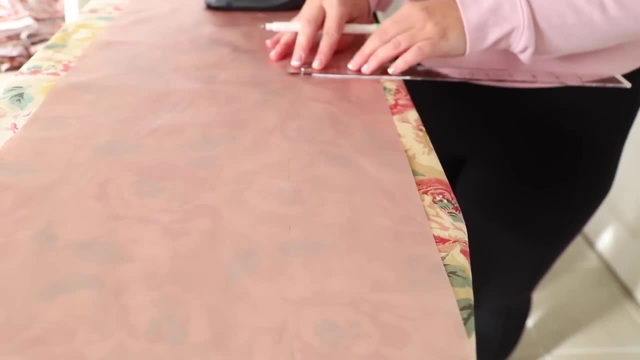 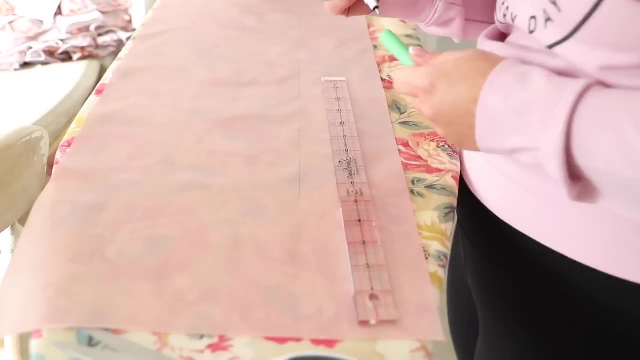 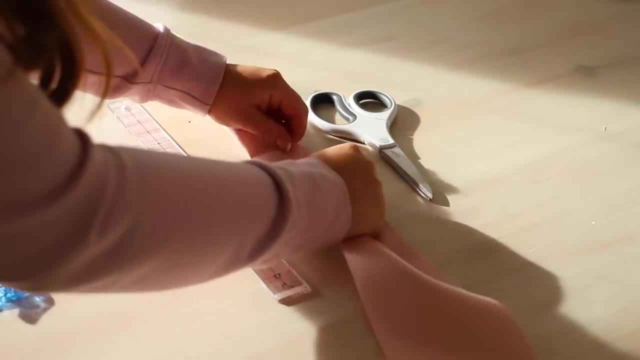 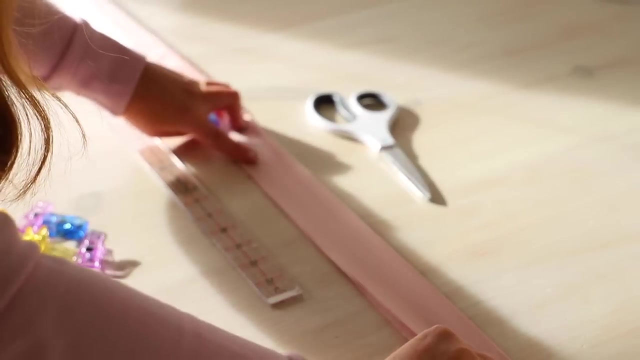 Measure out and cut a piece of fabric that is 35 inches in length and 3.5 inches in width. Fold your strip and fabric in half, with the right sides of the fabric facing each other. You can use pins for this, but I just find when I'm working with a silkier fabric, 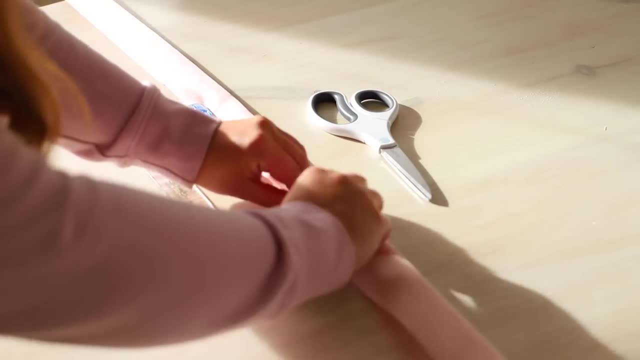 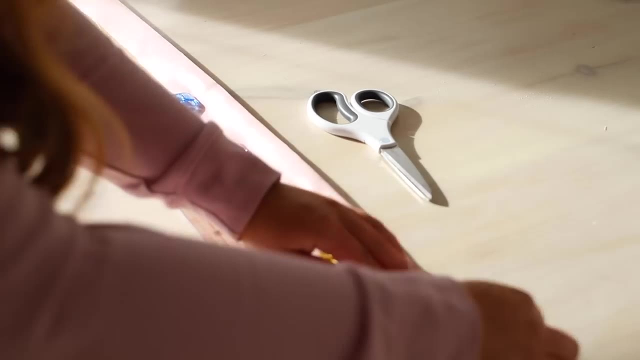 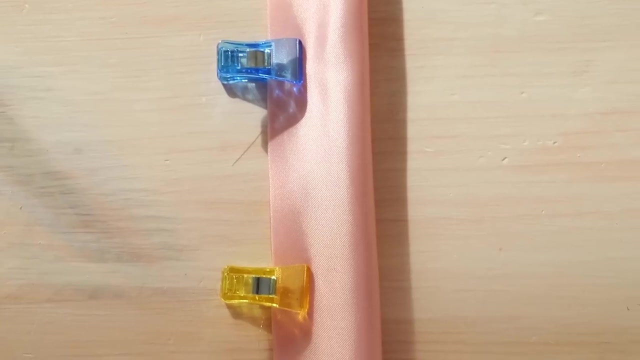 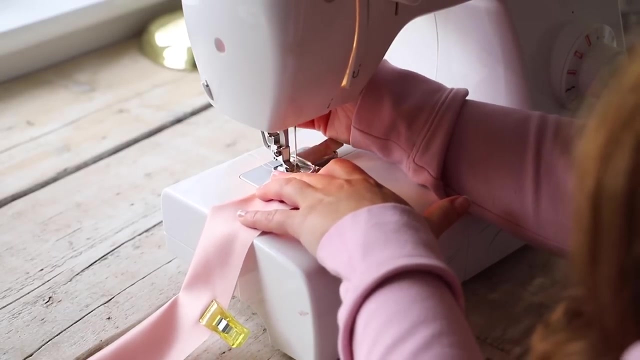 that the pins can mark it, so I'm just using these sewing clamps instead. Start at one of the ends of the fabric, Place it into the machine and do a straight stitch across With the needle. still in the fabric. lift your foot, press her foot, sorry. 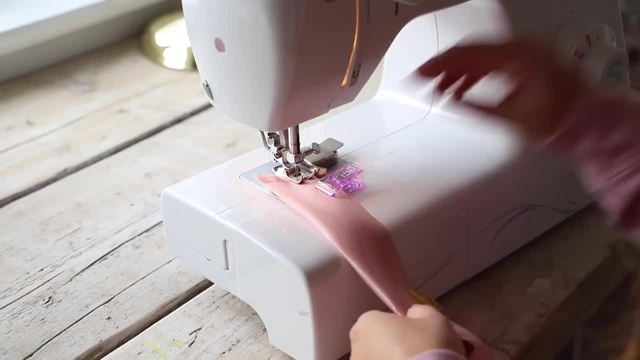 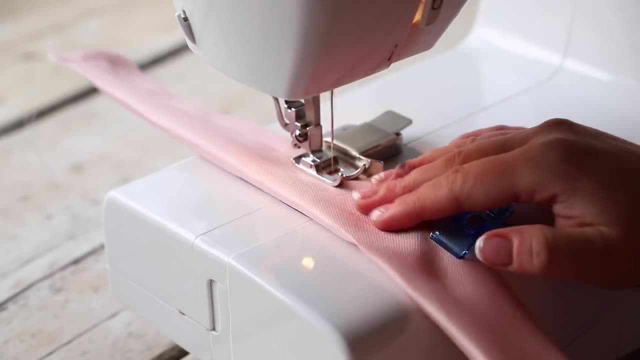 and turn it and then stitch down the length of your hair. roll When you get to the bottom, don't stitch across. You're gonna leave an opening so that we can stuff this, So where you put your pin and pin us in along. 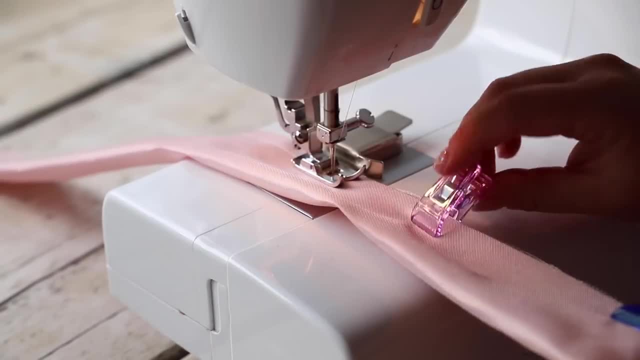 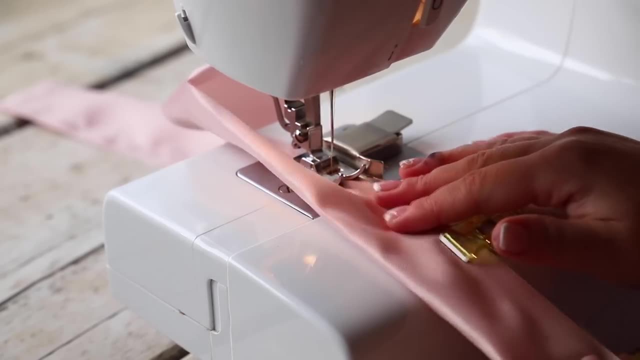 we're going to stitch this up. For now we'll just do a round off. I am just whale her. thank if you have one, and I just like what I get. I like thearnos from the Q&A a lot, so follow my SQL. we have the 911 on YouTube. 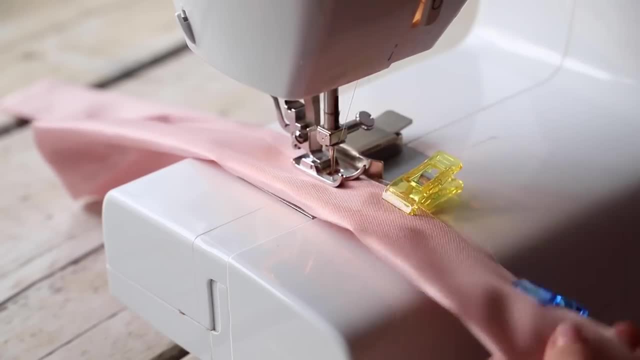 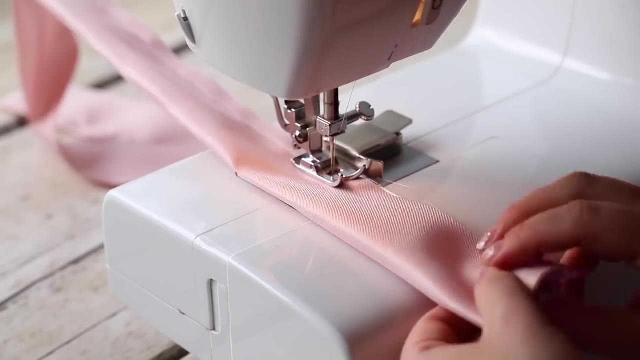 So the phone numbers: Z gets me the number. my number for помощil, Om A-U-M-V-I A-U. It's W, Right after you put your hand in the direction, let's get going pitches. These are. 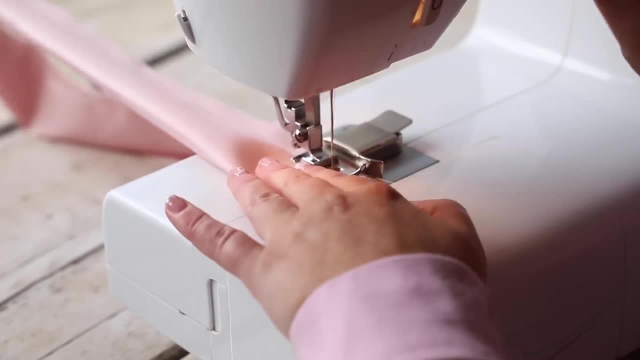 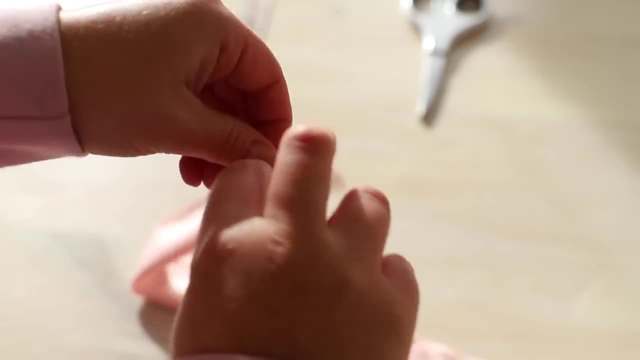 of course, family hair rolls, Abe, you go first. No, this one. it's much easier to use this safety pin to turn this the right way out. i didn't have one, but because this isn't too narrow, it's easy enough to pull it through with your hands. once i had. 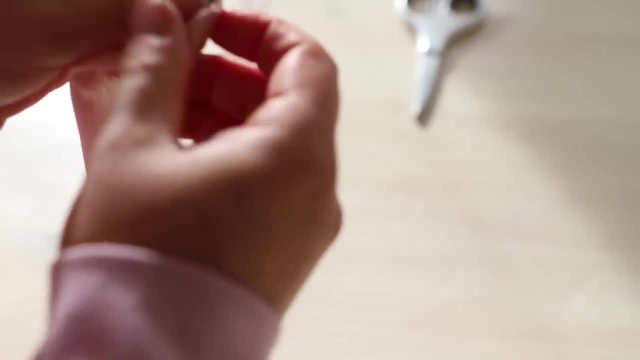 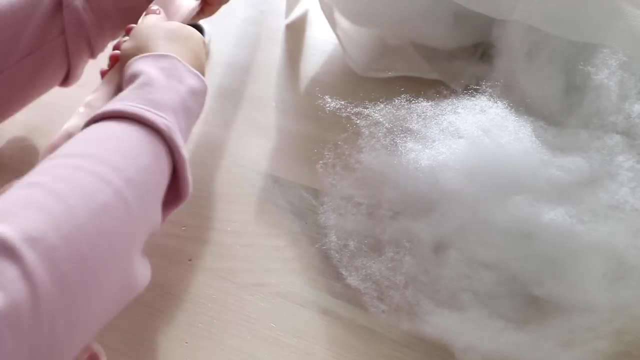 to pull the right way out. i then used some filler to fill it really tight and i packed all of the filler in. the filler that i'm using is actually from a cushion pad that i had. the hardest part of this project was actually filling up the length of tube with the filler, so take your time with. 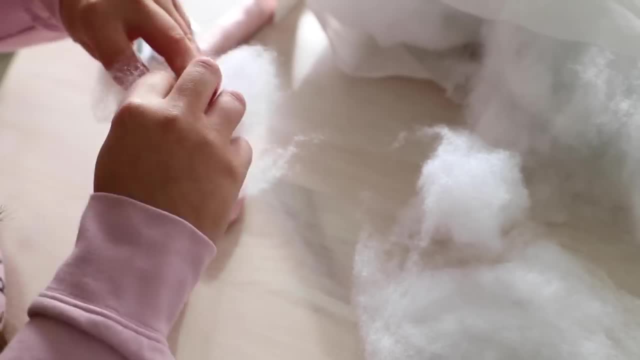 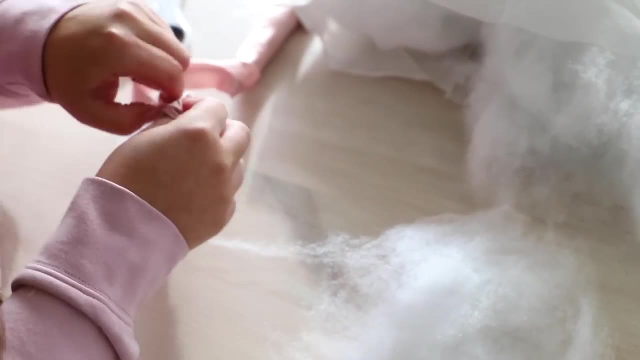 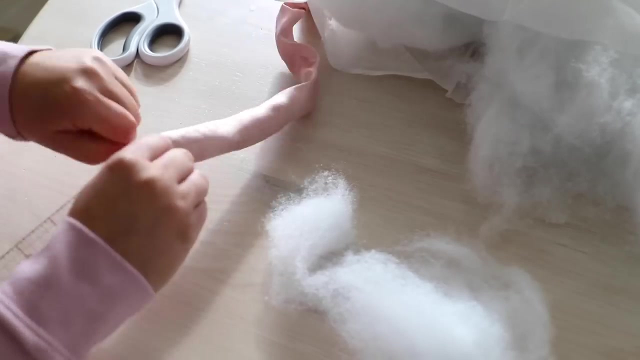 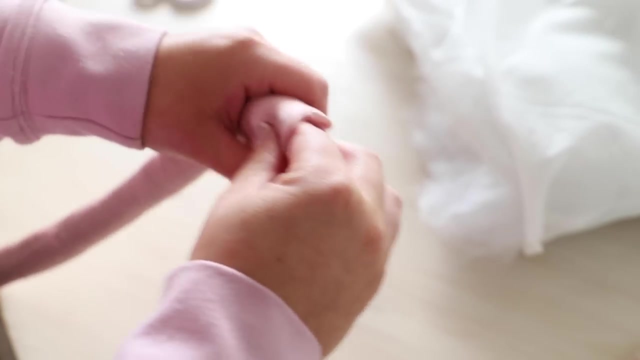 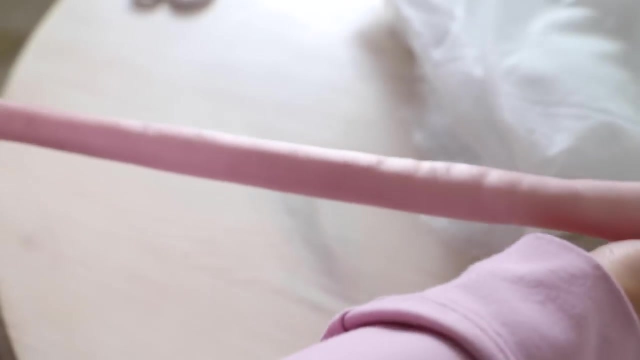 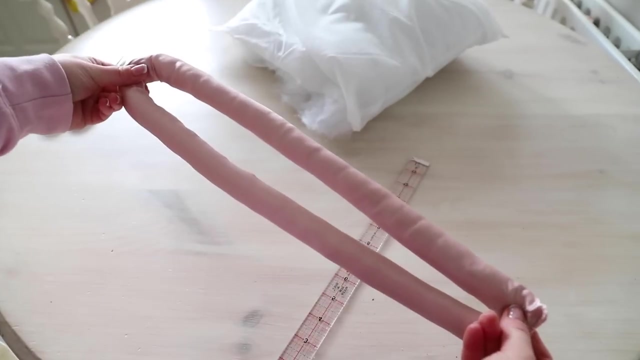 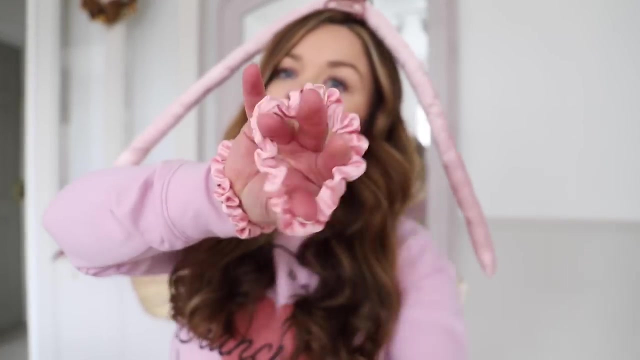 this and i just used my ruler to push it down to the end. once i got to the end, i tucked in the raw edges and i just did a straight stitch across to seal this up. here's a quick demo on how i use it in my hair. so i just use a claw clip to secure it to the center. 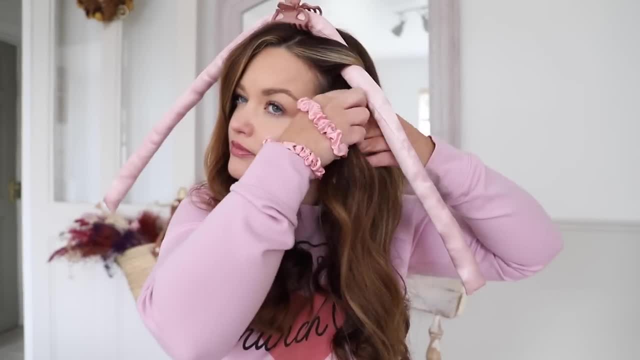 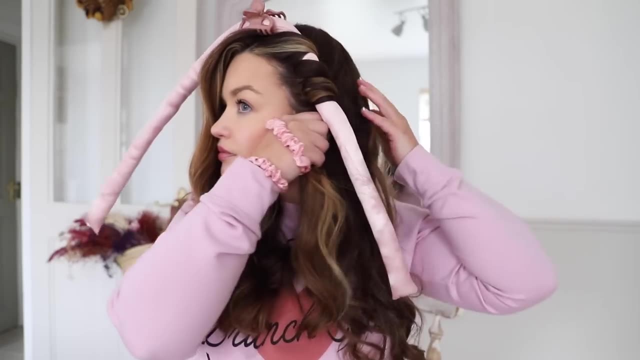 while i wrap it around- and i do it one side at a time- i start at the front with my fringe and layered pieces and then i just continuously wrap it around and tie a scrunchie in at the end. once the two sides are done, sometimes i'll tie a knot in the back. 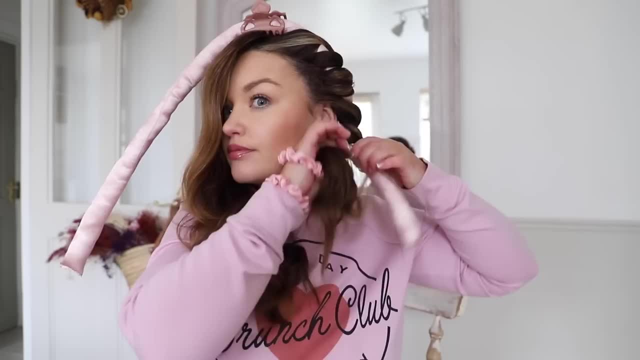 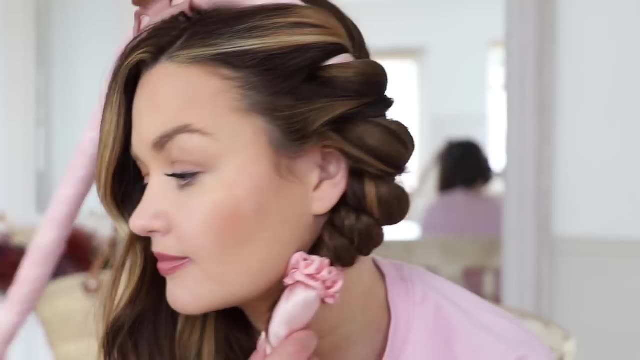 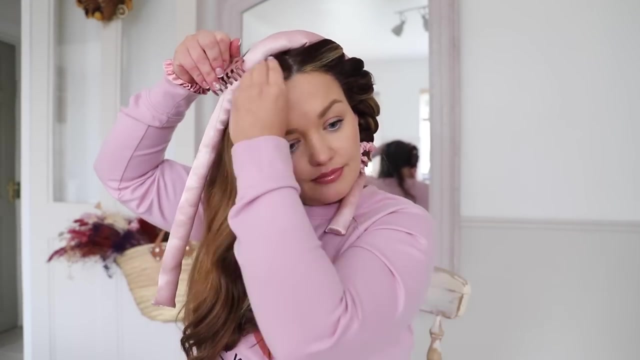 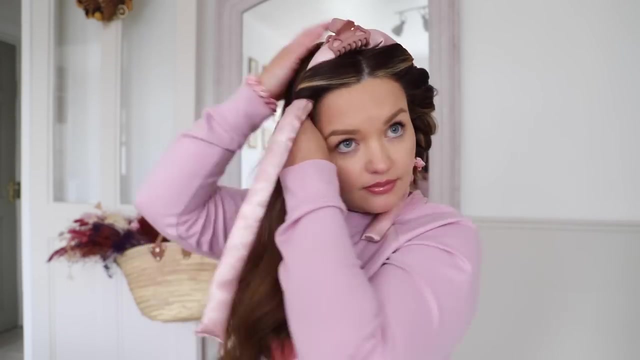 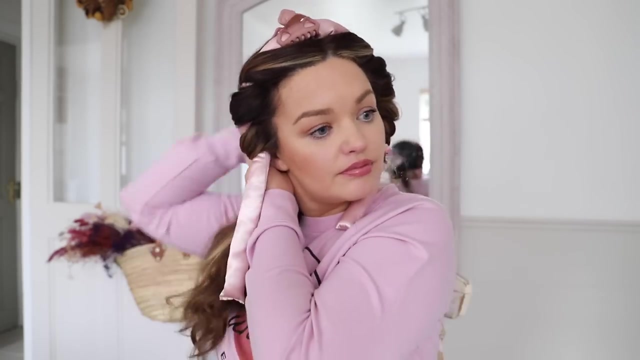 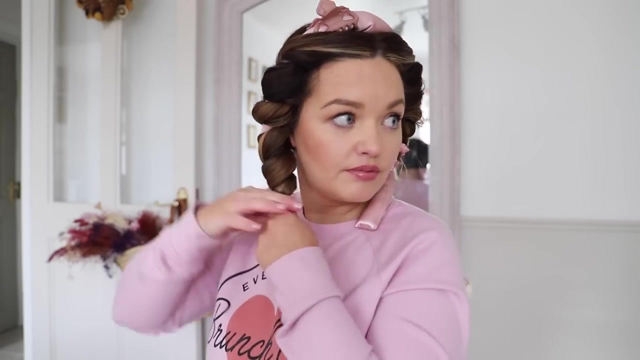 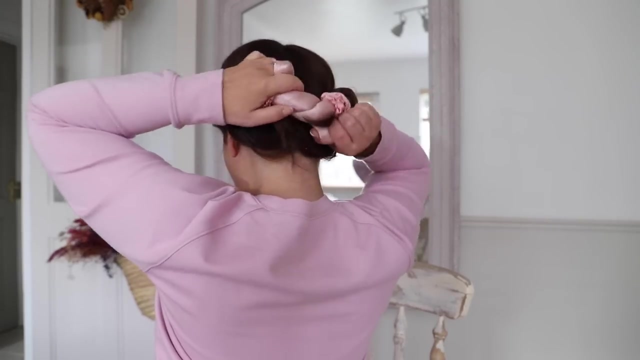 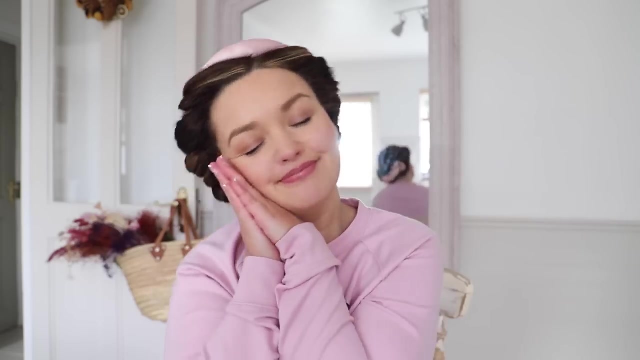 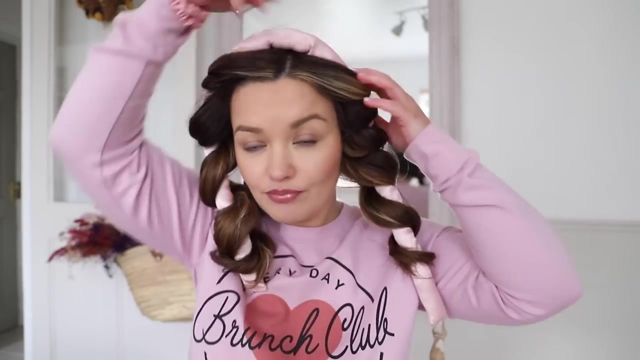 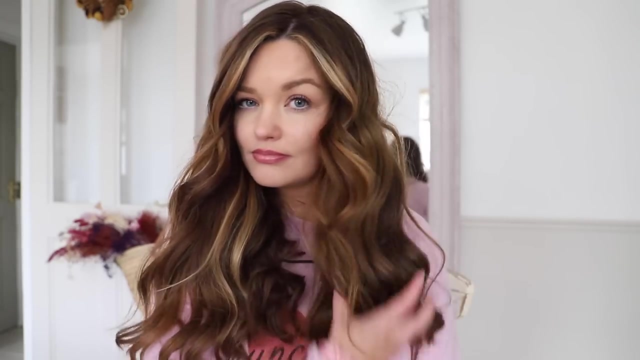 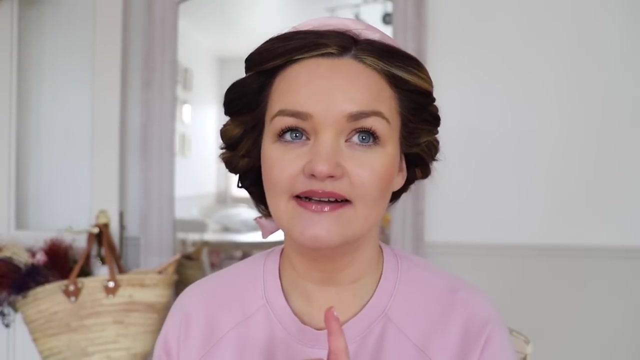 and then I sleep on this overnight, I leave it overnight and then I take it out the next morning. I take it out the next morning. Now I also want to share that you can. I have seen people do this with lots of things. 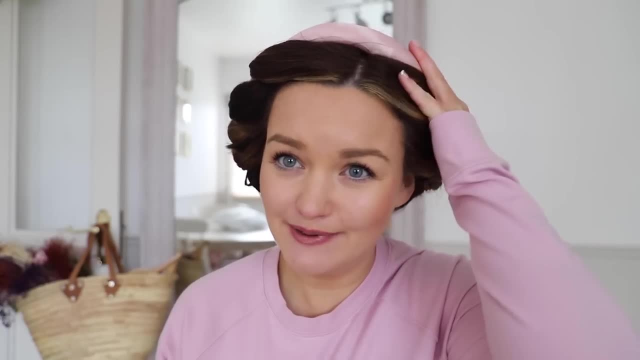 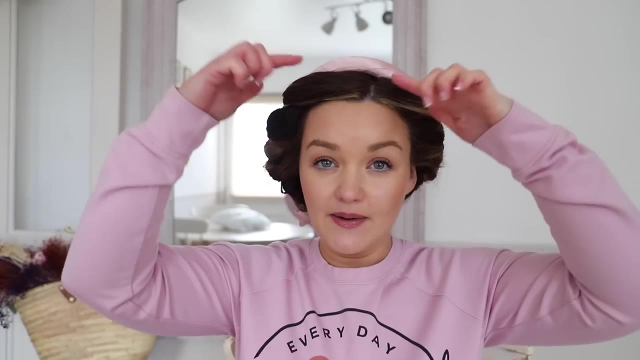 I've seen people do it with leggings. Nah, who wants to sleep with leggings on your head? I find these comfy enough to sleep in. Another thing I've seen people do is doing it the opposite way, but I just do this way because this is. 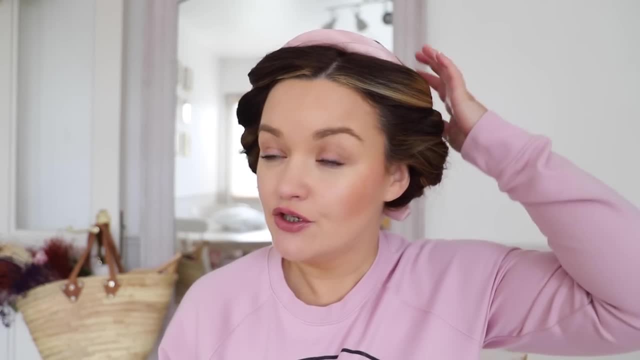 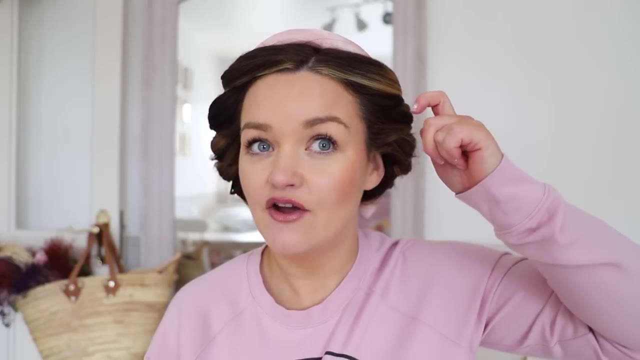 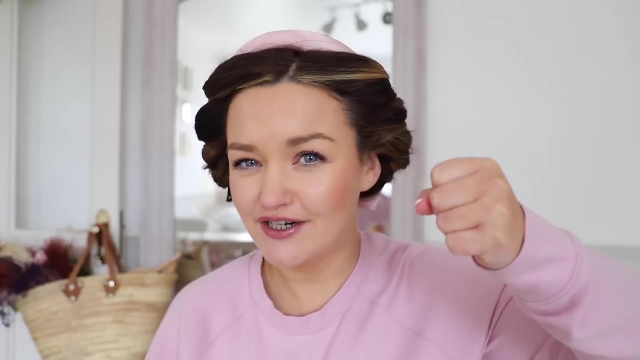 This is what works for me, so play around. The thicker your strip of hair, so do. thicker strips of hair is what I'm trying to say. for looser waves and smaller and more strands, for tighter curls. Am I saying that right? I'm going to take this out of my hair because my hair's already done. 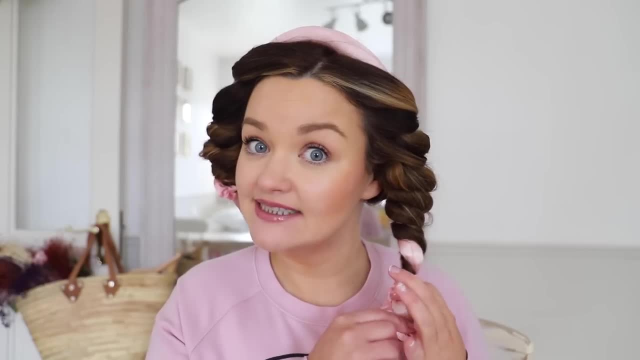 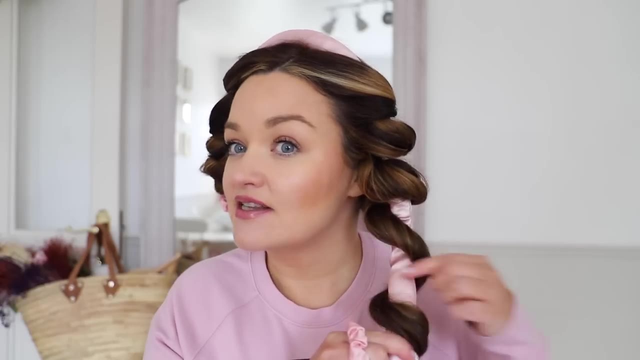 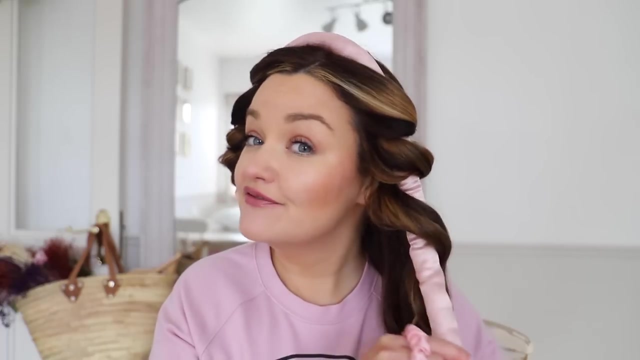 I've also seen people using dressing gown belts- So the belt off a dressing gown- But the only thing with that is, I'd say, it's going to cause more frizz in your hair. So I've seen like satin and silk fabric recommended for keeping your hair frizz-free. 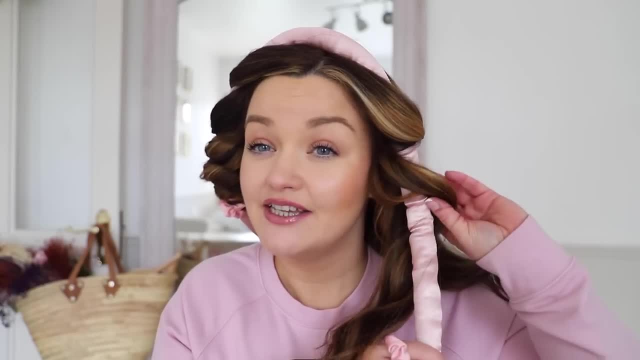 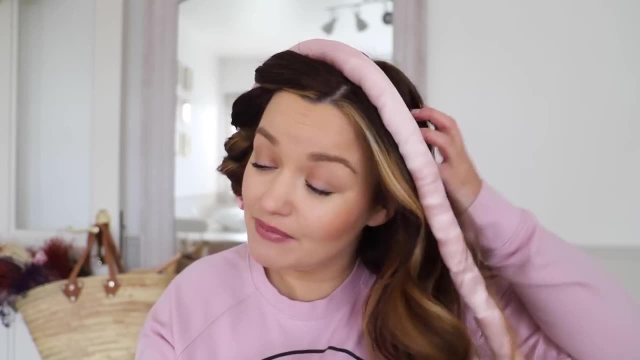 which is why I went for this fabric. But use whatever fabric you have. You could practice this with, like you know, bedsheet fabric, or if you have cotton length of fabric, you could use that as well. Whatever works for you. 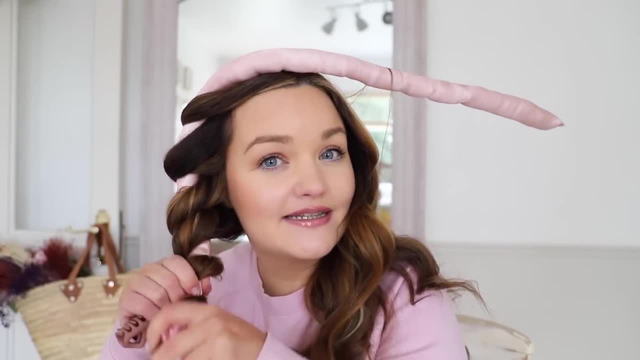 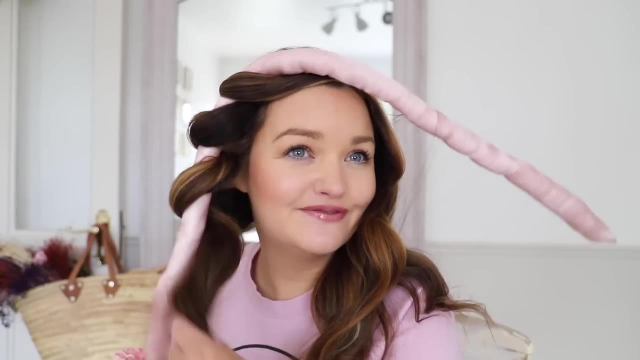 It also takes a couple of goes to get a knack that works for your hair type and your haircut. So don't be worried. if you do it the first time and you're like, oh man, my hair's frizzy. Do try it a couple of times to get a knack that works for you. 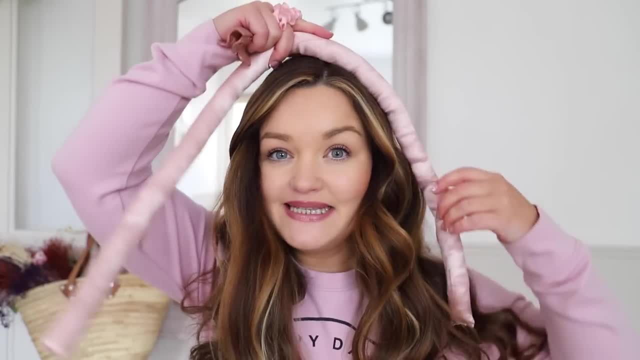 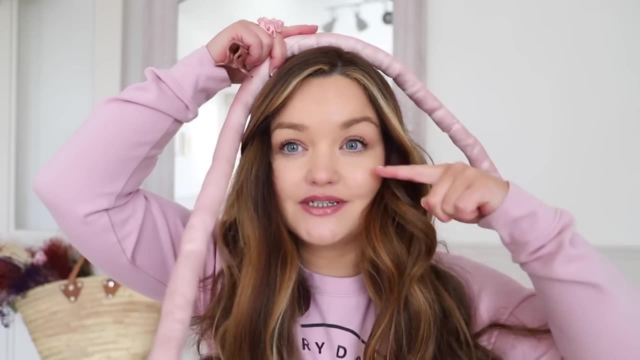 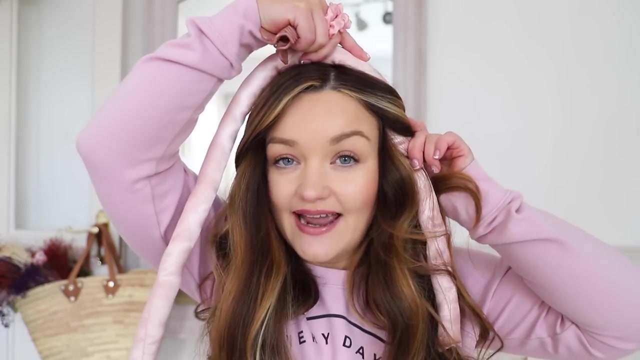 The knack that works for me is when I'm sticking it in So eye level. I want my first curl- so, for example, this one, to be eye level. So when I'm doing this front section, I make sure it's around there. 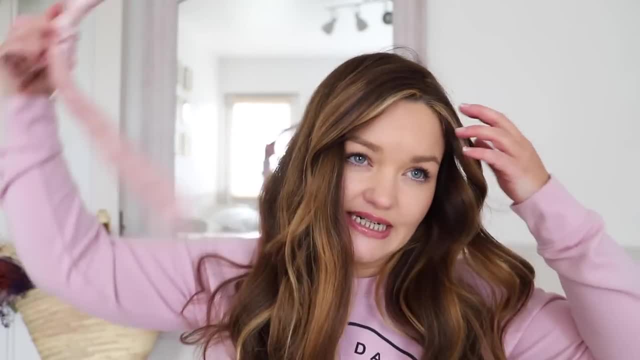 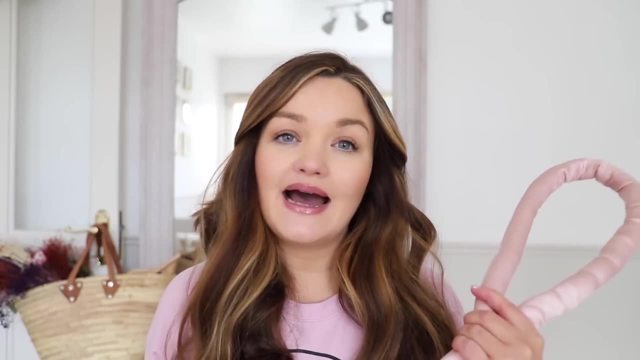 Does that make sense? Sorry for looking through the viewfinder. I know that's probably really annoying, but I've no mirror. Well, behind me, You could also do a shorter one if you had shorter hair, But I like having the little bit extra because then you can tie it behind if you want it. 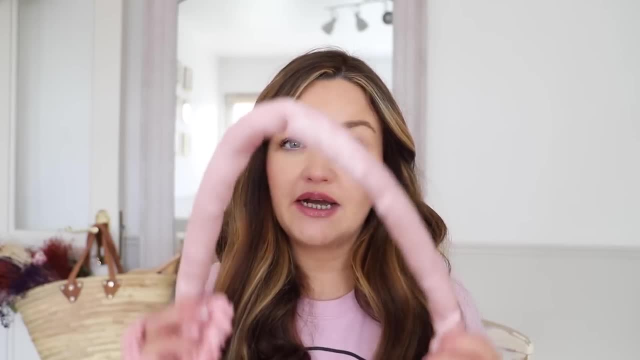 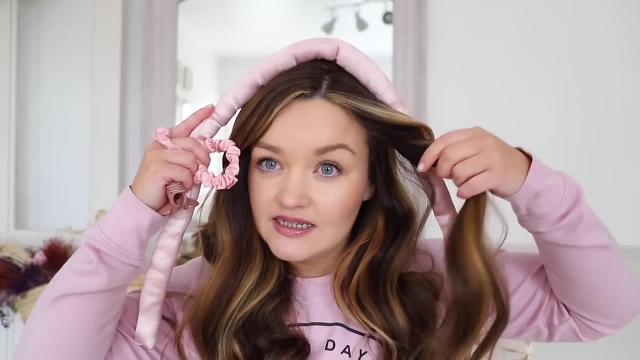 So yeah, it does work for short hair, but just bear in mind where you position the curls. So if you have like a bob and you just want a few curls, start up here at the eye level And then keep going until it's down. 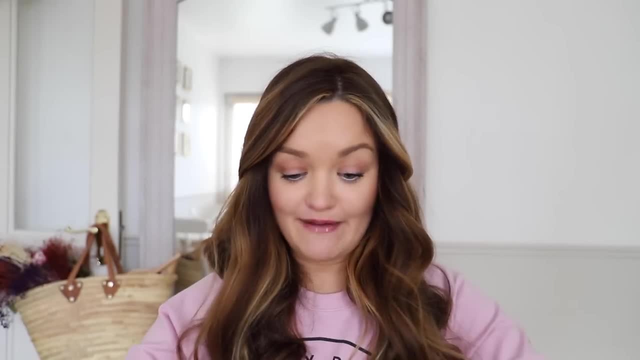 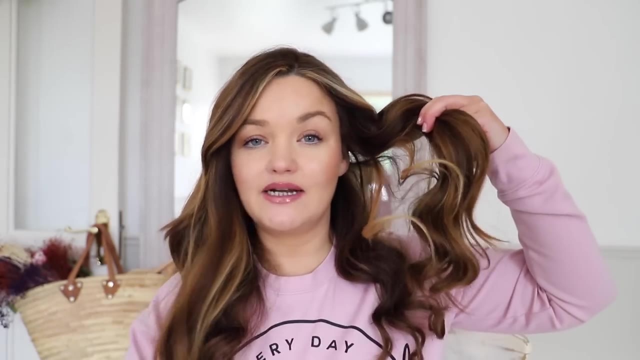 I'm really bad at giving hair tutorials. This ain't my jam. I also have a tutorial if you want to make scrunchies on an older video as well. Don't worry if the ends are quite curly, because it will fall throughout the day. 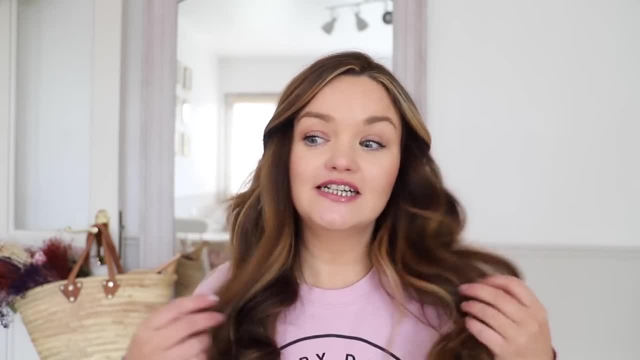 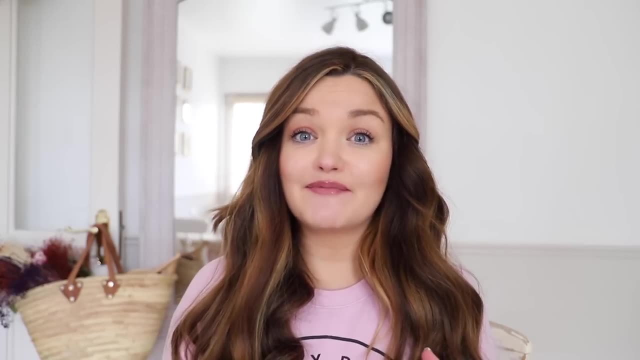 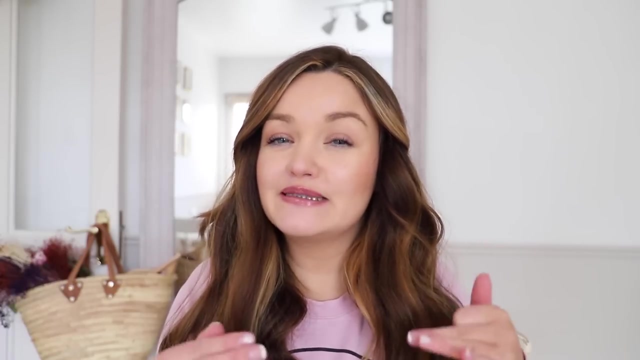 And sometimes I'll just spray a bit of like texture spray in it just to give it a bit of fluff. And also, if you do it the first time and you're like, oh my god, my hair is huge, you could tame it with a curling iron, which defeats the purpose of the heatless curls. 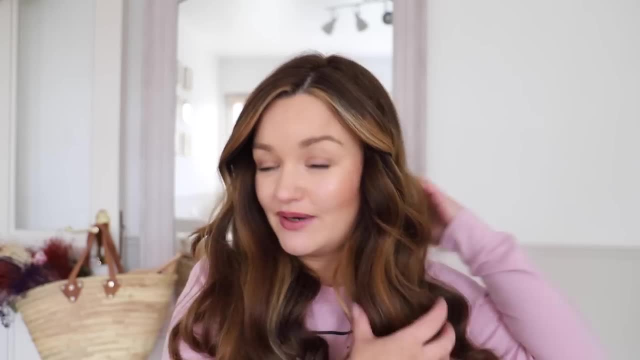 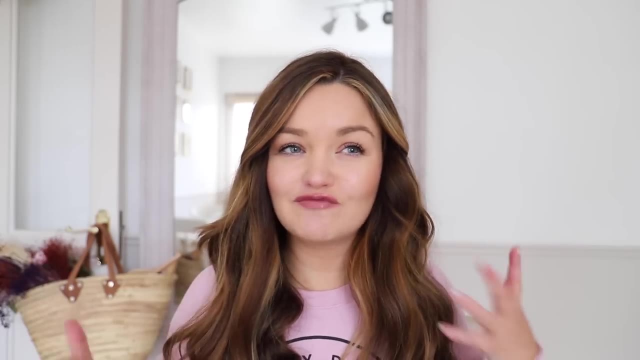 But if you do need to tame it, it's kind of easier when your hair is already curly, to hold the curl and then just throw in one or two curls around the head just to give it a bit more. how would we say, maybe, definition structure. 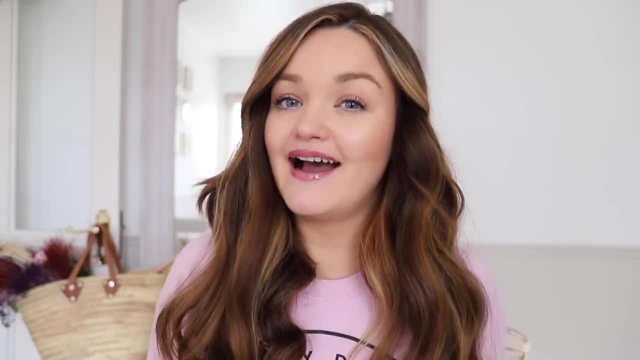 I don't know the word. Anyway, let me know if you try it and if it worked for you. And if it didn't work for you, I'm sorry, And if I gave you a bad hair day I'm extra sorry. 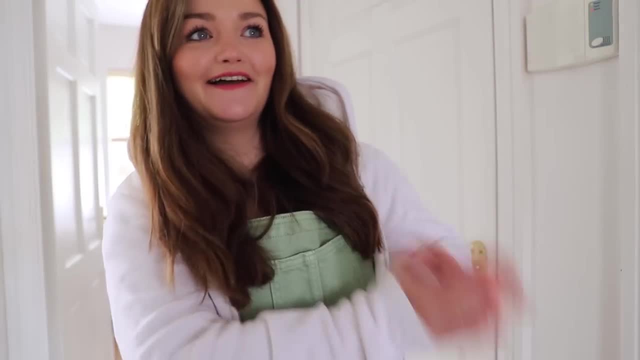 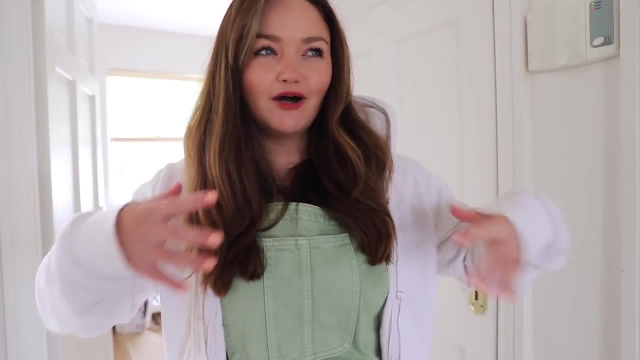 Why is it typical? It's been lovely and sunny and warm And the moment I go to make myself some, I want to make some loungers easy to sew. I'm hoping they'll be easy to sew. I want to make some loungers for my chairs out in the background so I can sit and chill and be comfy. 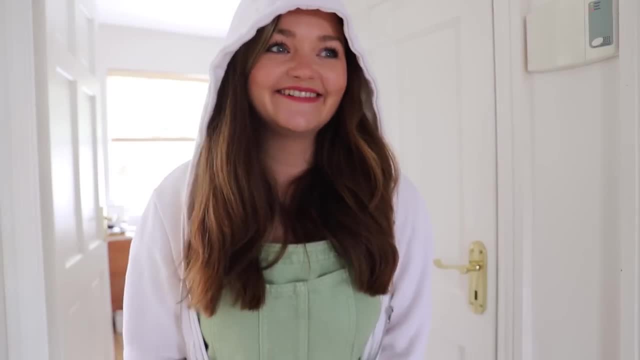 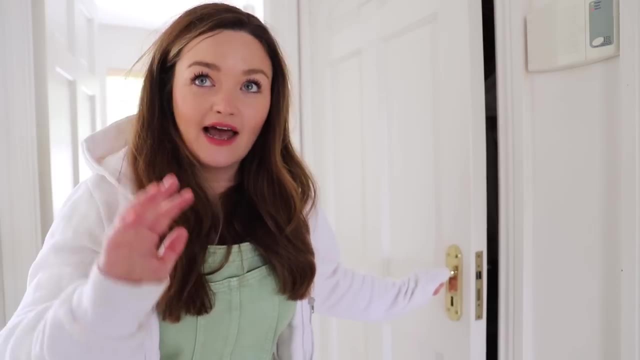 But it's gone cold And I think it's due to rain- Typical. Anyway, let's go into hot press. I know I have a blanket that I want to recycle. the fabric Hands up who has too many blankets? Who has too many blankets in the house? 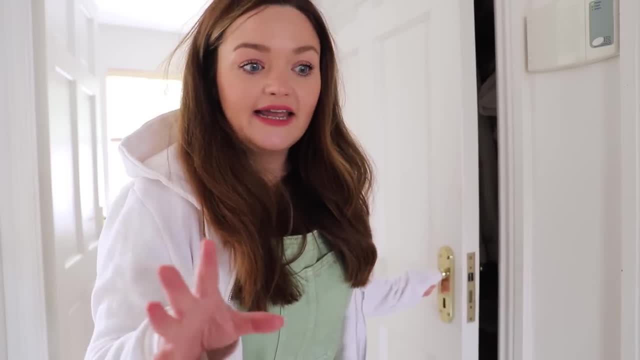 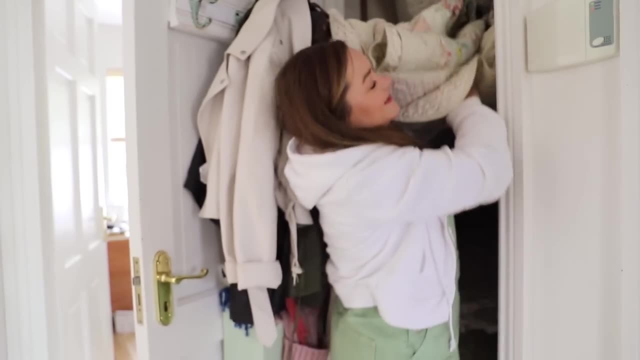 Bit of a blanket buyer, bit of a blanket hoarder. I have to stop myself. I have a blankie. Oh, look at this, it's taking me hot press. Anyway, I have this quilted blankie, but it's actually from Penny's Hun. 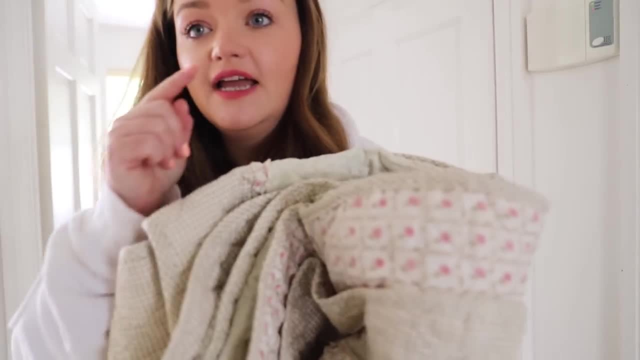 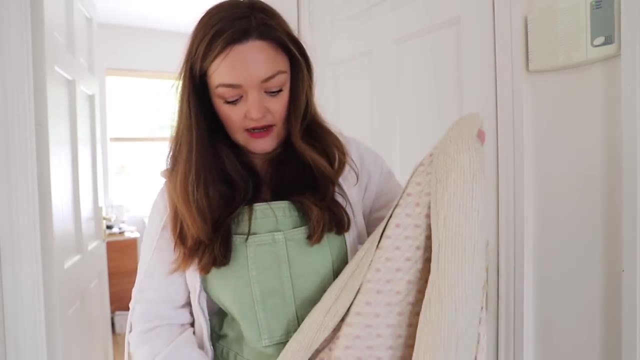 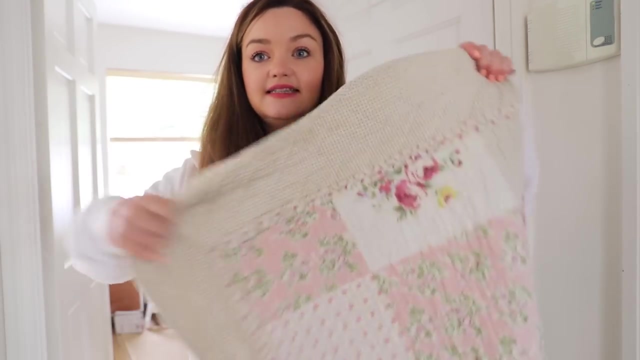 I got this years ago. I do love it, but I have another one that's similar. I think I got this on sale in Penny's Primark if you're in the UK. One side is this, The other side is this: 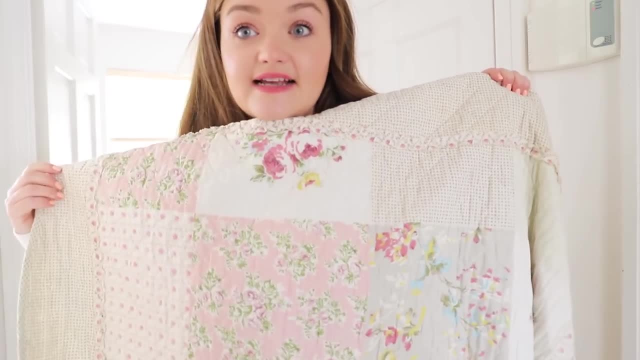 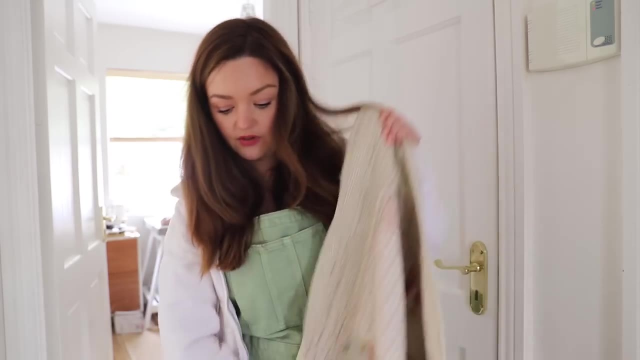 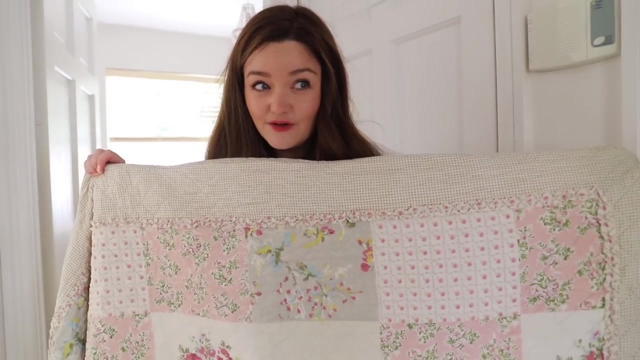 Like I think I got it on sale for 10 euros years and years ago, But I'm going to use this material to create- I should have enough for two. Yeah, because it's. I have loads of fabric Like I probably even have enough fabric to do cushions. 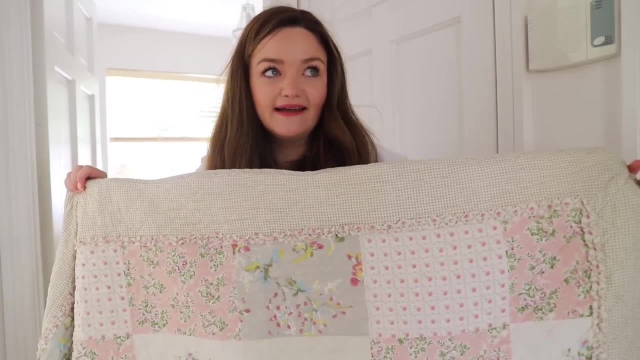 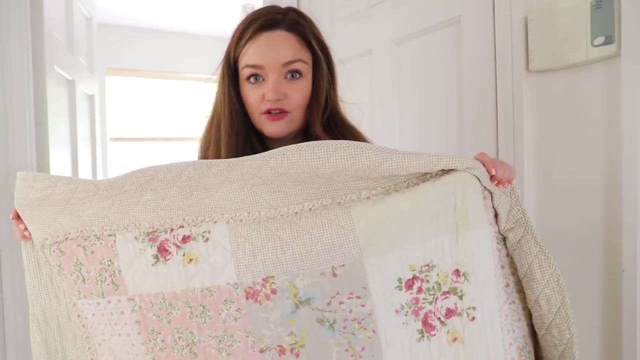 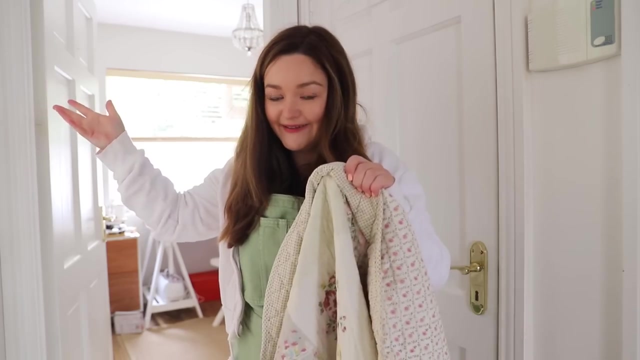 Like not bean bags. but Yeah, I'm going to recycle this And We're going to make some outdoor like seat pad cushions. Hope that makes sense. Sure, you'll see. anyway, First thing I got to do is measure. 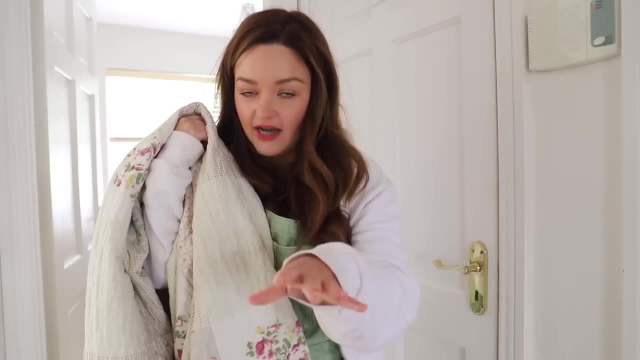 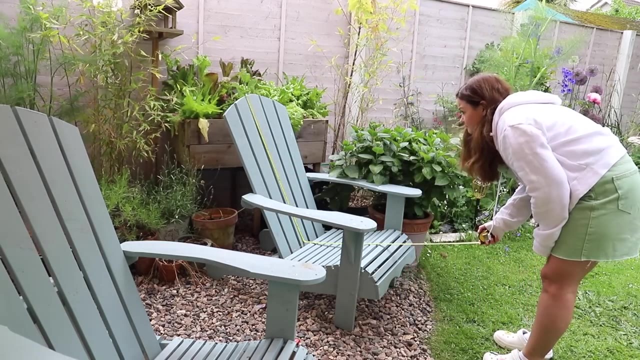 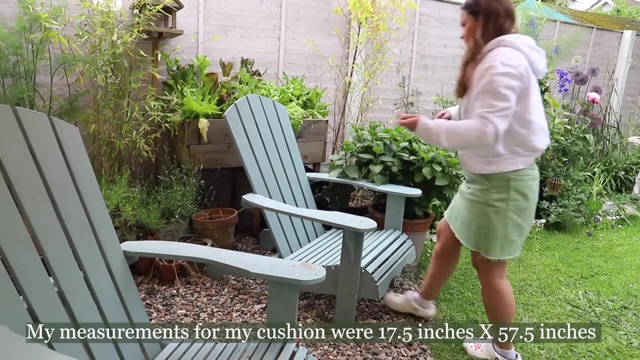 Measure the chair, And then you'll get an idea of what I'm doing. Let's go So. I began by measuring the length of the chair to determine how long I want it to be, And then I also measured the width- And I'm also lolling at me- using a good old builder's measuring tape. 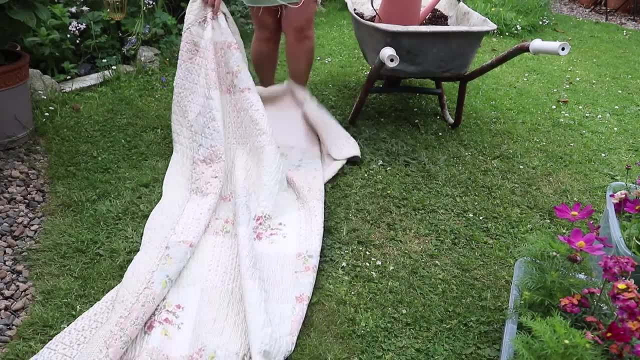 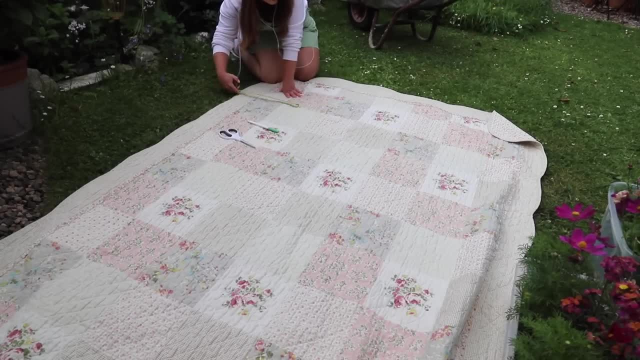 and not my usual sewing tape. But sure, here we are and it did the job. I then transferred the measurements onto my old blanket And then I cut the first strip out. Once I had the first strip out, I went back to the chair and I just laid it on it. 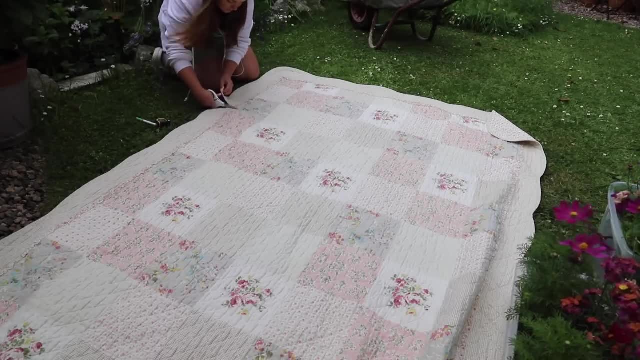 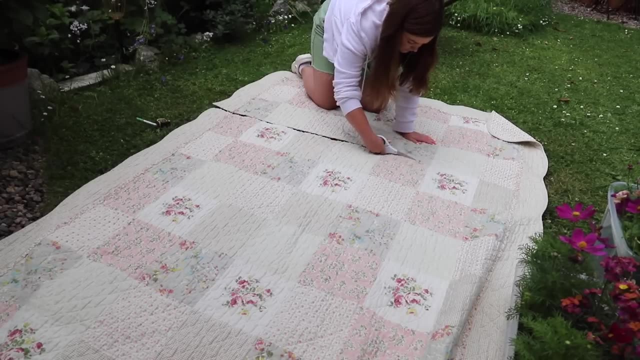 to see like: was it too big, Was it too wide? Now, I did leave an extra half an inch for the seam allowance, So once I was kind of happy with that, I then used that first piece that I cut as my template. 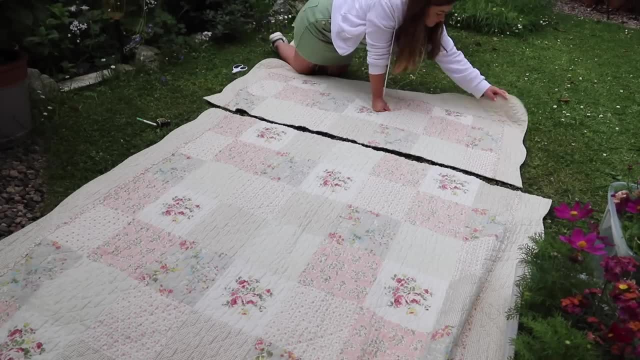 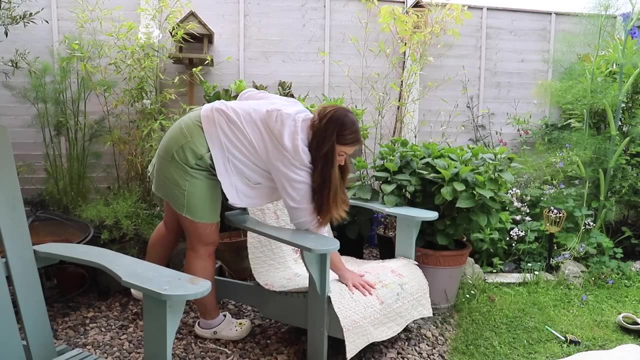 to cut out the rest of the pieces. So you're going to have a front piece and a back piece, and then we're going to make handles. The handles are totally optional, but if you want to kind of carry this or fold it over, 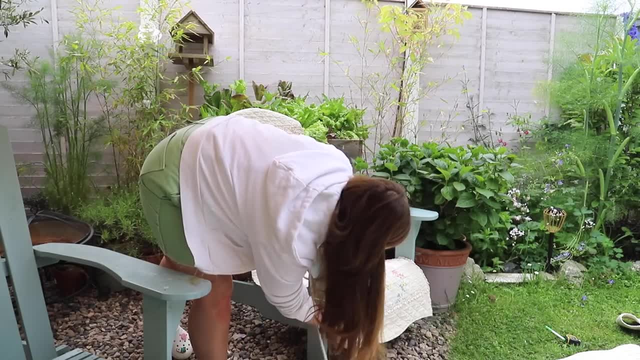 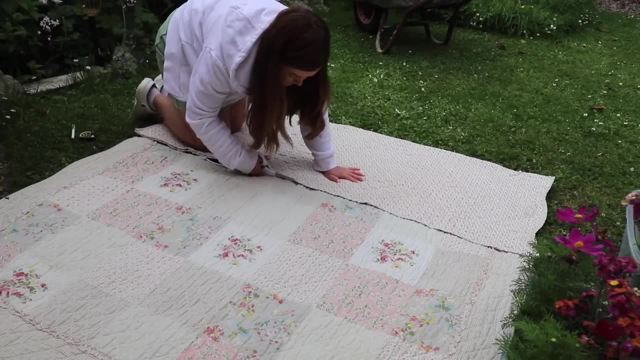 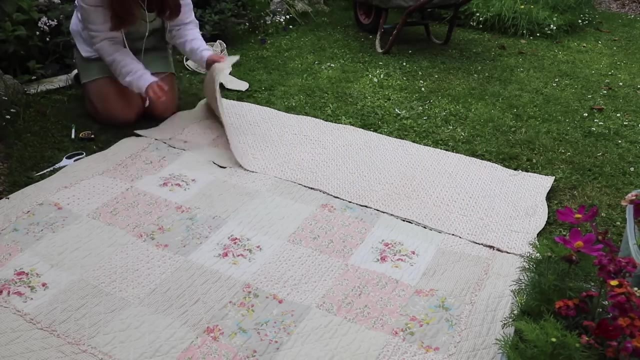 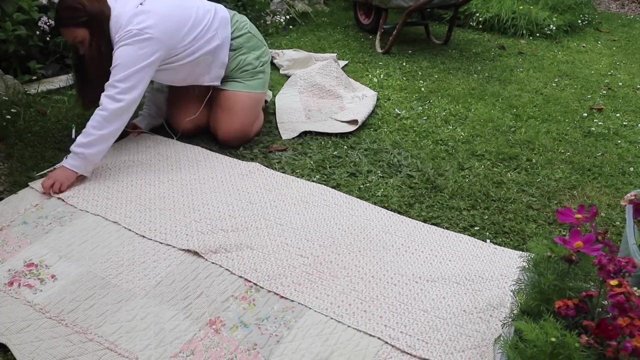 and have it as like a little portable picnic cushion. then the handles are really cute. I've had this up for about three weeks now and I'm just going to have the front part and the back part folded And then I'm just going to turn it over. 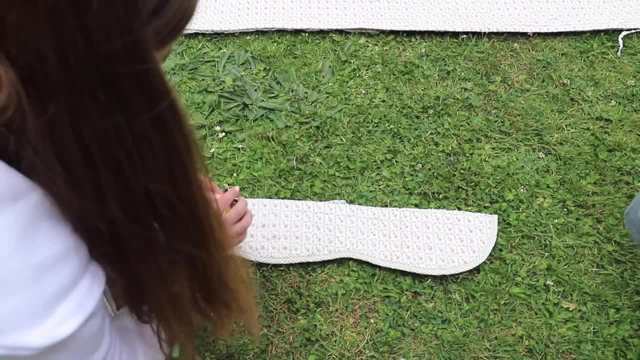 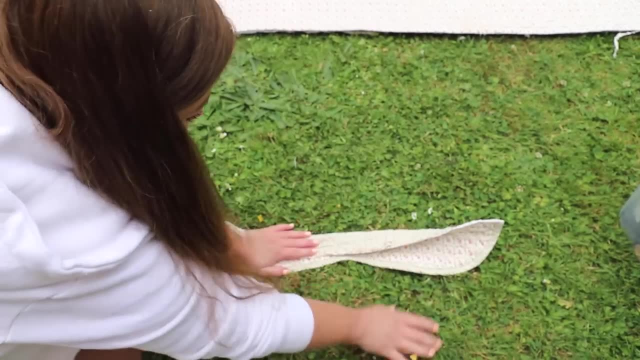 in a little bit of quilting, and I'm going to do that. So I'm just going to fold and roll here and there, and then I'm just going to fold over and fold over and over again. I'm going to take my knitting bag. 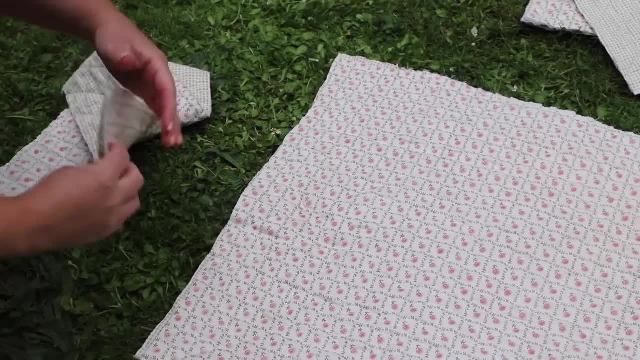 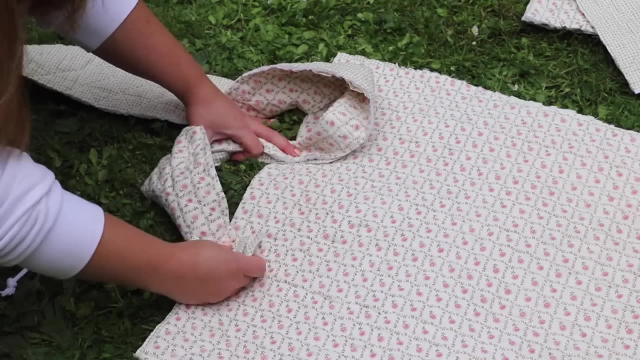 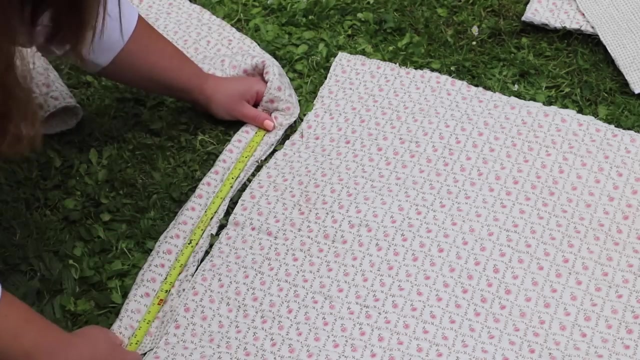 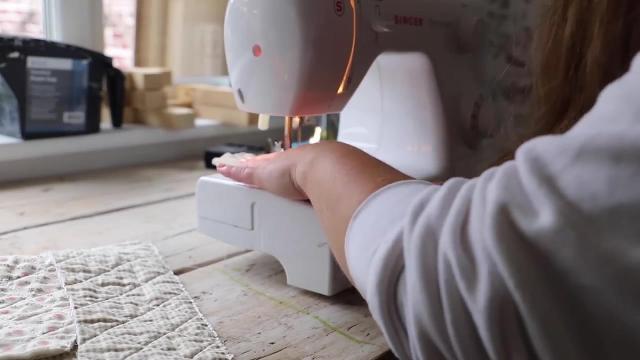 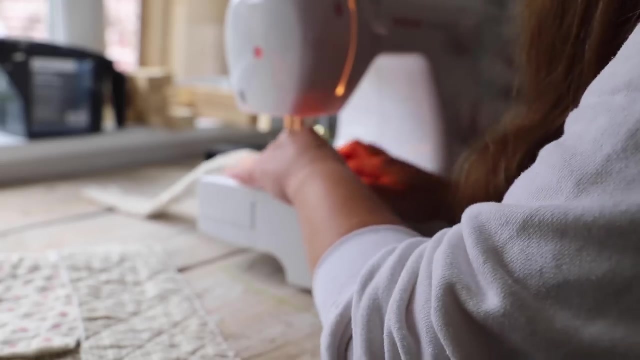 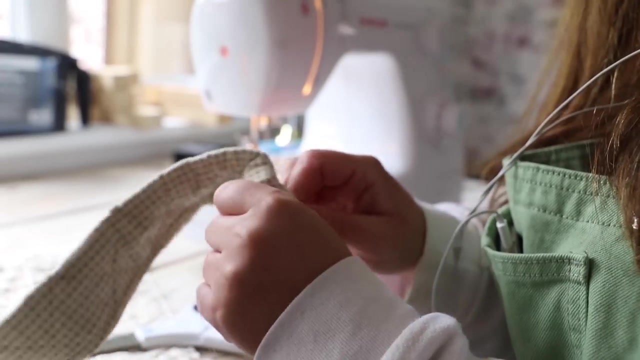 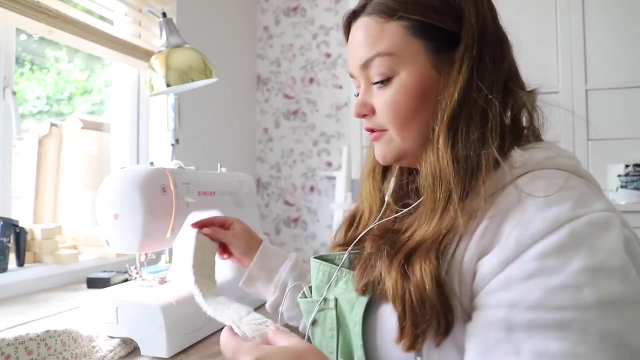 and I'm just going to flip it over like this. Thank you for watching. I just want to share a mistake I kind of made because my fabric is too thick, So you would have saw me just there fold this in half, put it through stitch at the end. 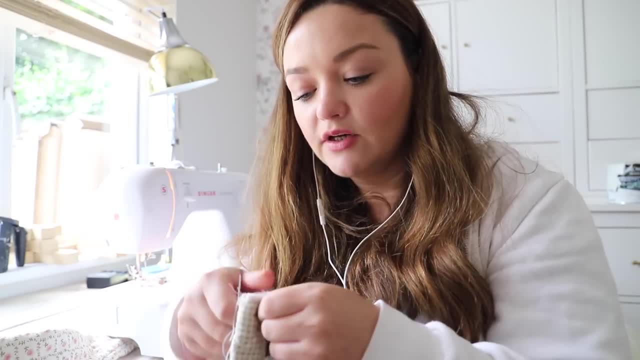 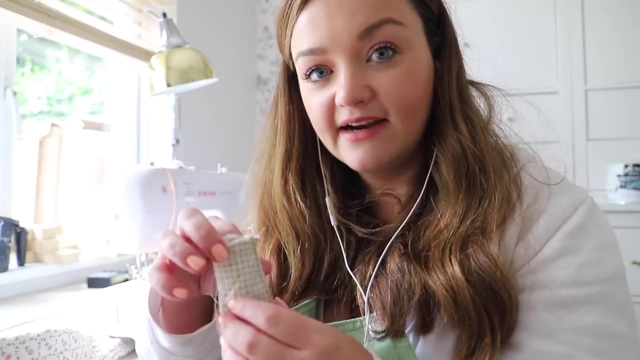 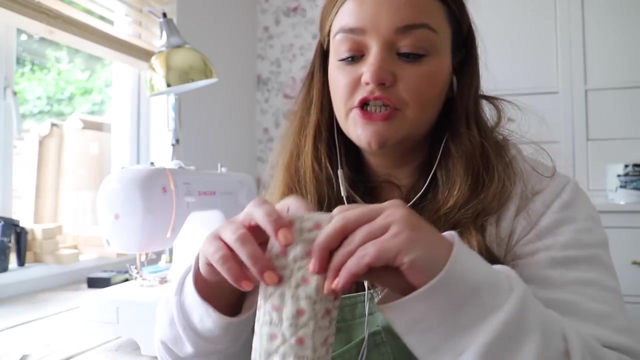 and then the idea would be to pull it the right way out. But because my fabric has padding in it, because it is a kind of quilted material, this is too thick and your girl can't get it through. So I sandwiched two of the pieces together, left the ends open, because these ends are. 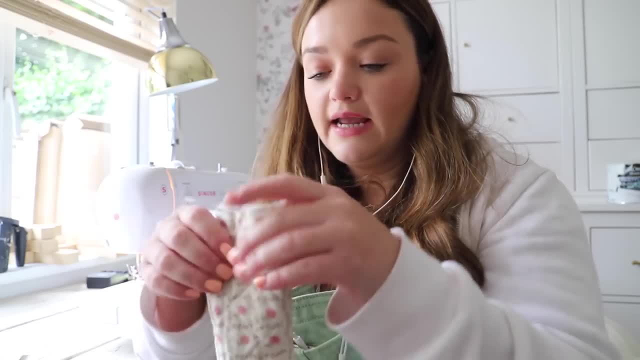 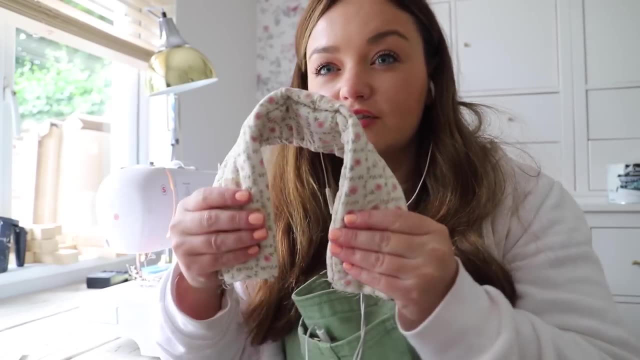 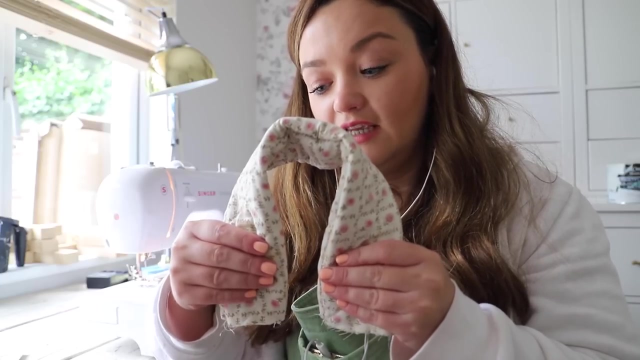 going to be tucked into the piece anyway. So I have- I just need to iron this so I have- a thicker strap that is going to look like this and it's going to be on either end of the cushions. This is also optional, because the reason why I'm sticking a little handle 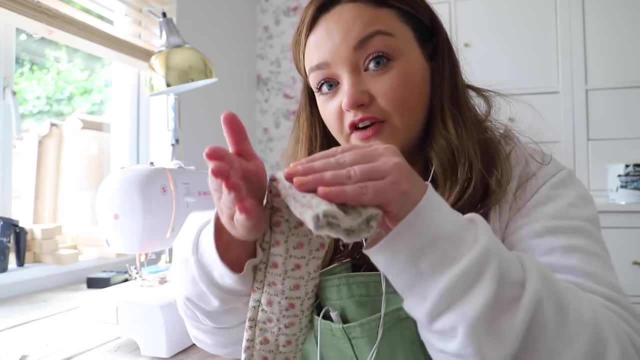 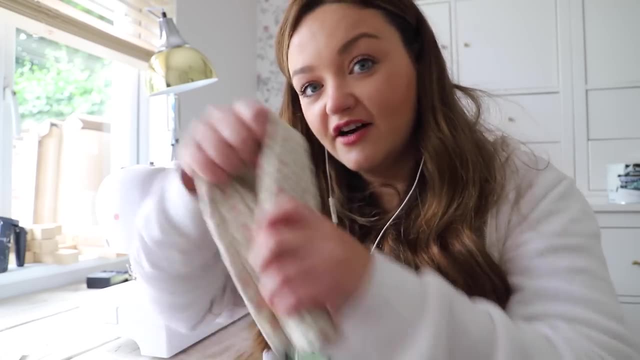 on is so that you can fold the cushion over on itself and you'll have two handles, and then you can pick the handles up and walk off with your little cushion, So it's like a portable kind of cushion. Well, it can be a picnic cushion as well, so you can fold it in half. 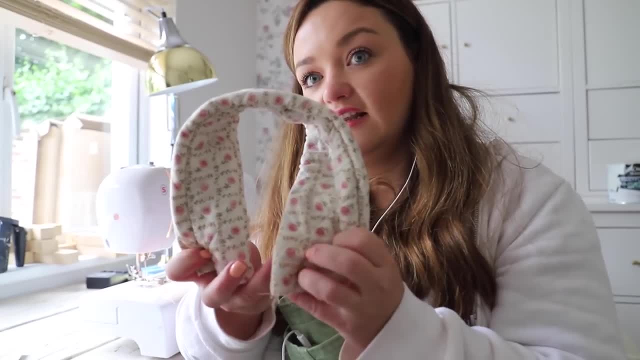 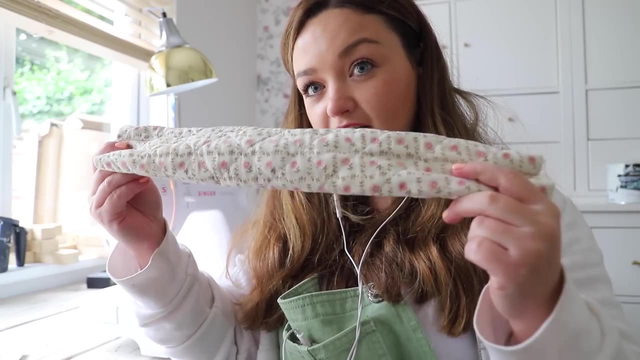 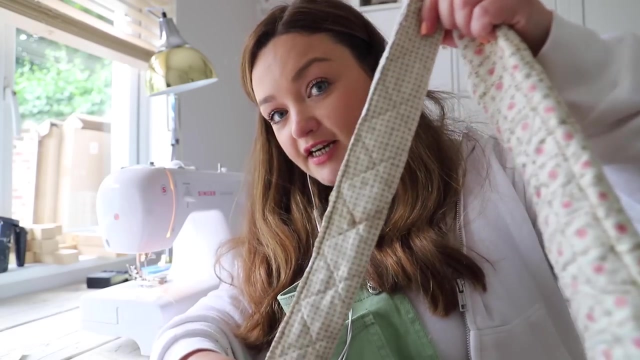 So that is, these will stitch in to the thing nice little grip on it. It's still, I'd say it could do with being a little bit smaller, But I want to use this material. So that method does work. but if your fabric is too chunky, no. 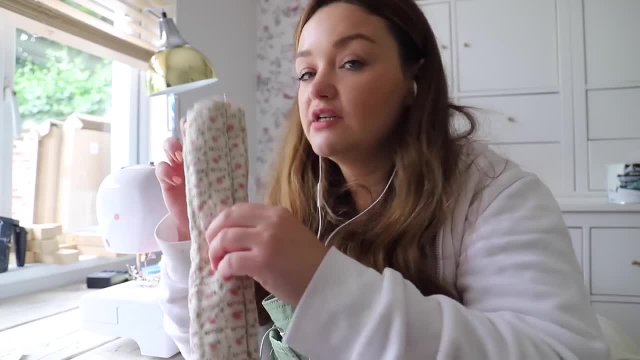 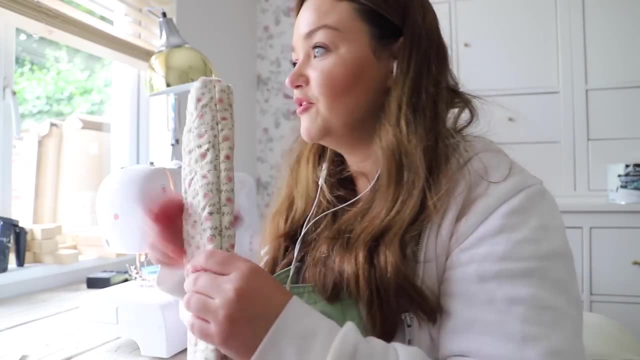 So I have some. I do have some more scrap of the edge of the blanket that I can make. Actually, I'm making two cushions. I need to make three more of these, So here I am just making the straps, the final way that I've done them. 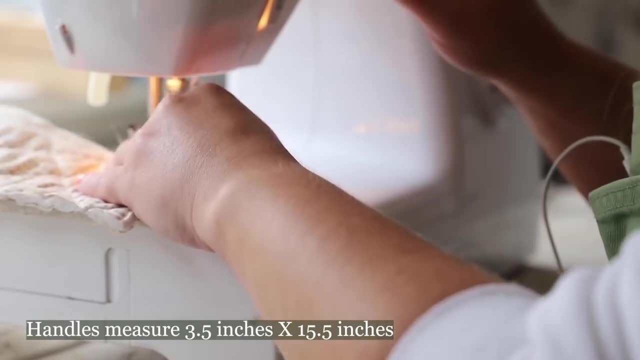 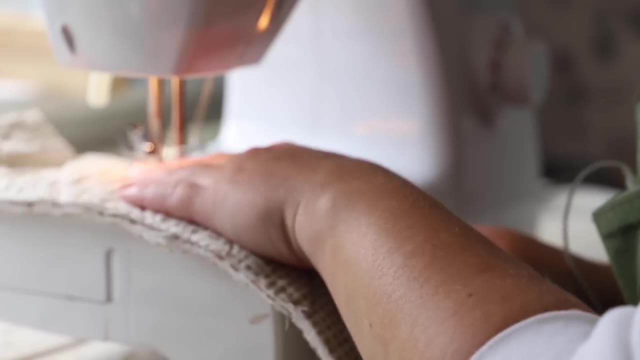 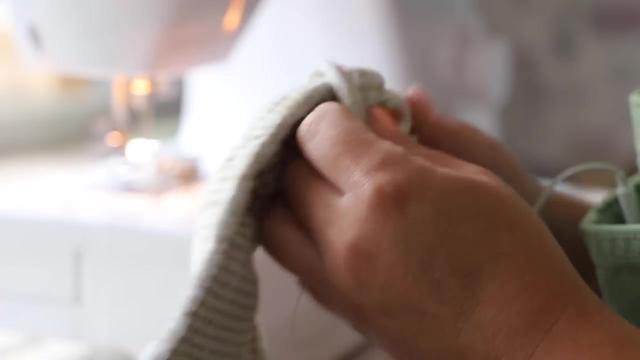 So I did the right sides of the fabric facing each other, a straight stitch down one side and a straight stitch down the other side. I turned it the right way out, and you'll also see that I did a decorative top stitch. When material is kind of chunky like that, I think this top stitch just gives it a lovely finish. 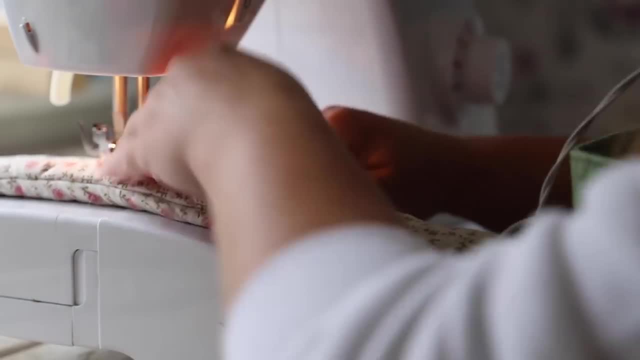 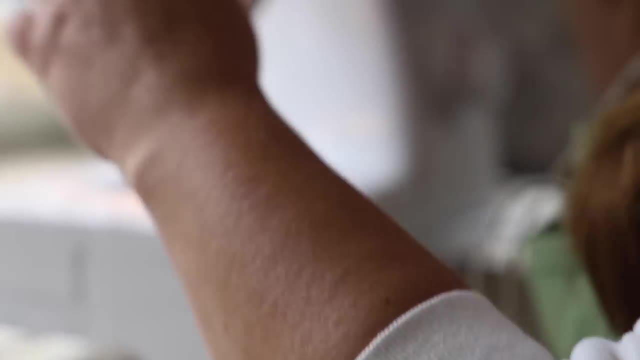 So I'm just gonna go ahead and join the main line in the top and the bottom, And this is what I did for the bottom, And this is for the top and the bottom, the bottom. So now I'm going to stitch these up and I'm going to fold them in half. 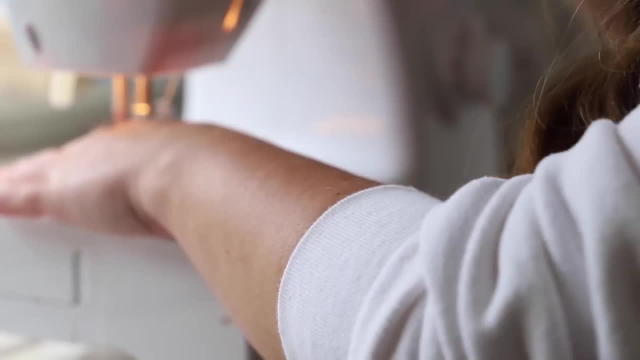 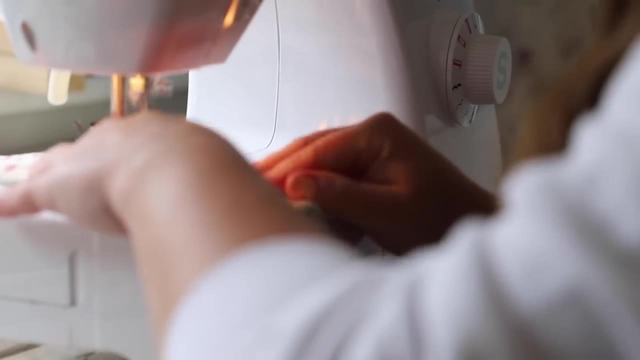 And there you have it: a beautiful and simple gift box for your kids. All right, So now I'm just going to take this little spike of the fabric and I'm going to see what this doesn't look like. I'm going to have to give this a little bit of a stretch, and that's a good idea. 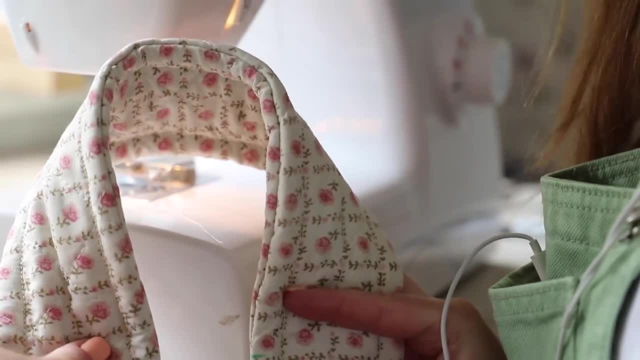 We're going to have toودo it, I'll cut it back. I'm not going to cut the ends off. You wanna see it? Yeah, Okay, just watch carefully to see how I put the handles. make sure that they are facing inwards so that 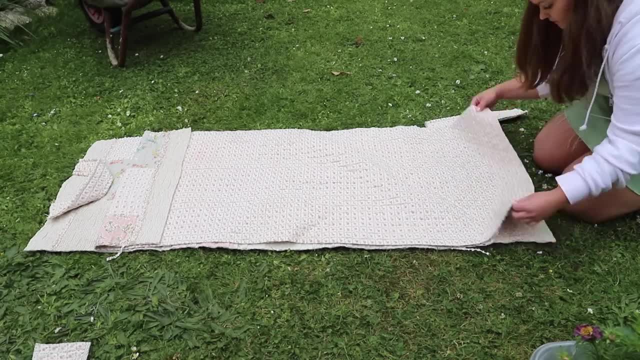 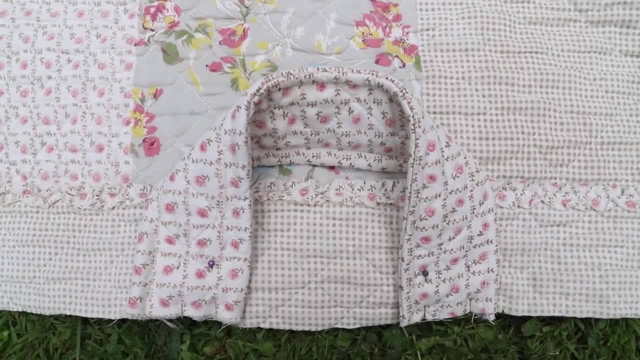 when we stitch all around this piece and you turn it the right way out, the handles are going to be on the outside. I know that this can be confusing for beginner sewers, because I used to get confused by this as well, and so this is how you position the handles before you stitch around. 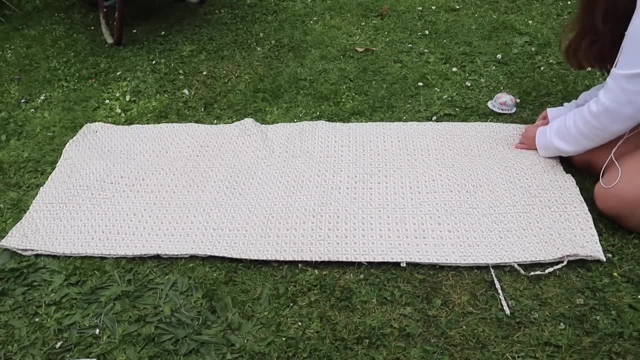 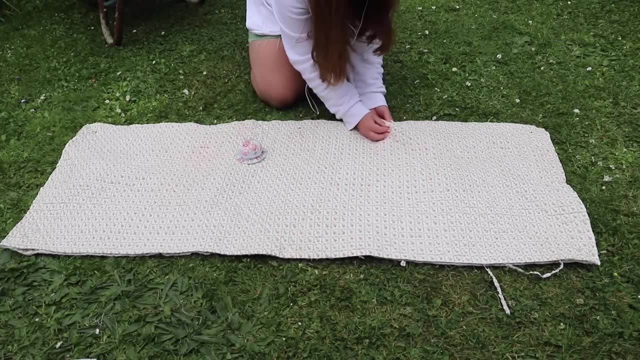 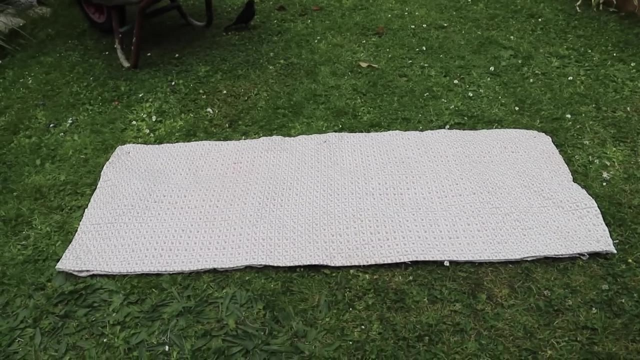 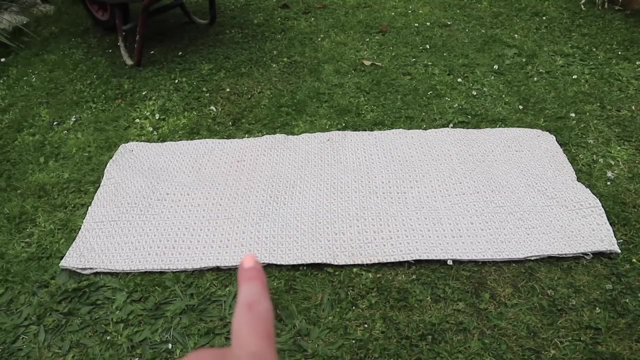 Mr Blackbird is very intrigued by what I'm doing. I don't know if you can see him in the corner. he'll come in shot now. So do leave a gap on the side so we can turn this the right way out. so I'm going to leave a decent size gap, maybe like two hands full, and I'm going to 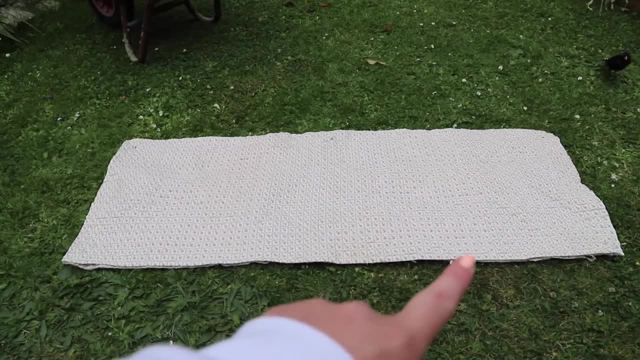 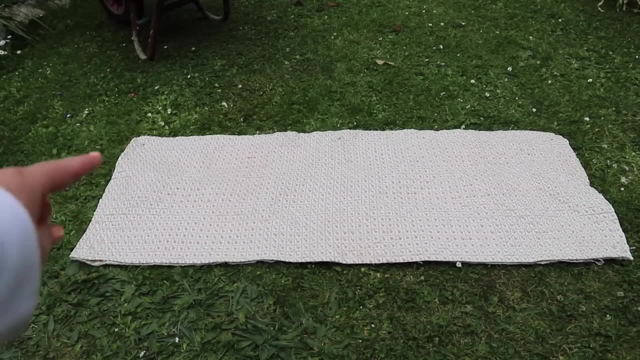 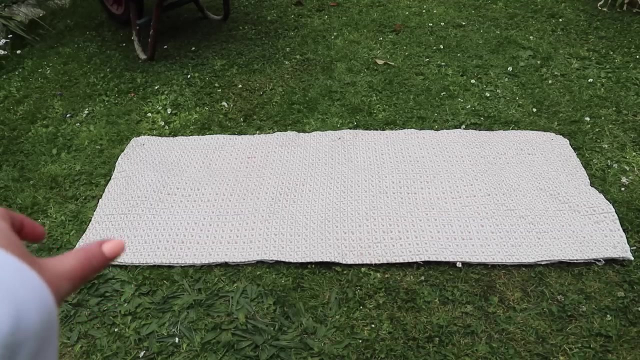 stitch all the way around, leave the opening, turn it the right way out when I'm going over the handles, because the fabric is quite thick, I might just do a bit of a reverse stitch when I go over the handles and I'm going to leave a good half an inch seam allowance on this, so I'm going 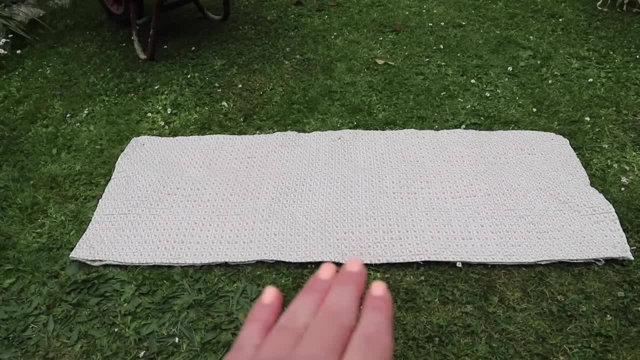 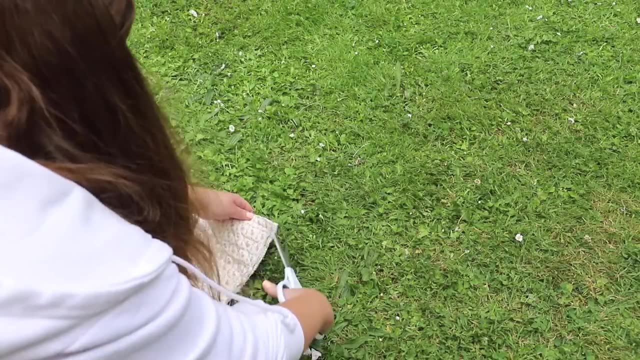 to take it to the machine, and I'm going to go all the way around, leave the gap and then we're going to flip it out and then we're going to stuff it. Just before I turn the fabric the right way out, I'm just clipping the corners and I'm also just taking off any excess bulky material on the. 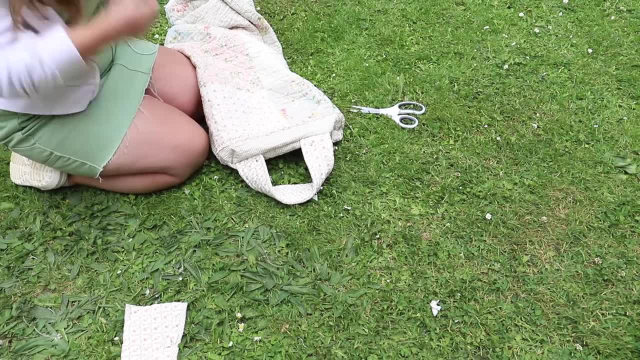 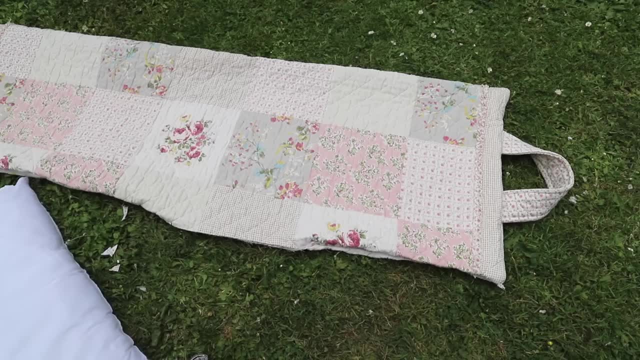 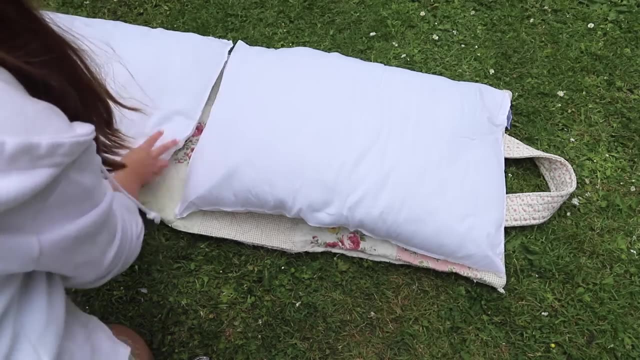 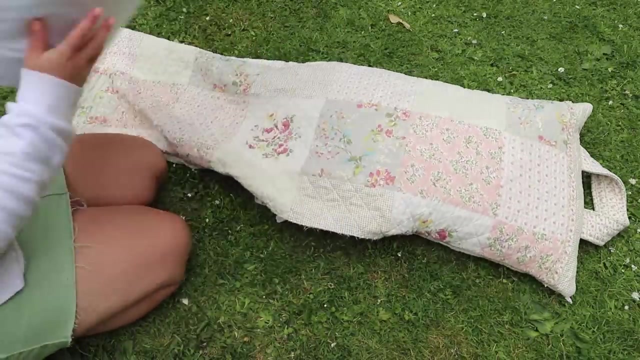 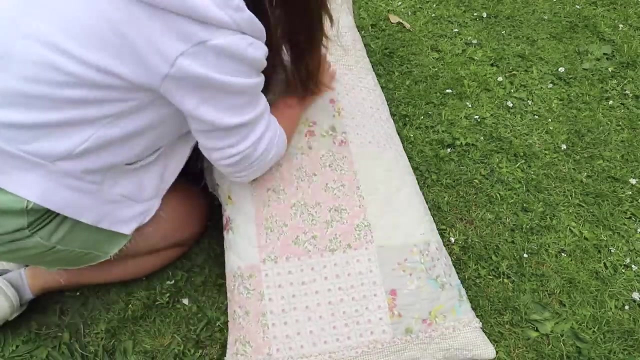 sides. just be careful not to snip too close to your line of stitching or you will weaken this seam and your stitch could unravel. I do some of this to make sure I don't lead any way down, and that's it. I'm putting the two loops together at the bottom of the fabric. I'm going to tuck it in like so. 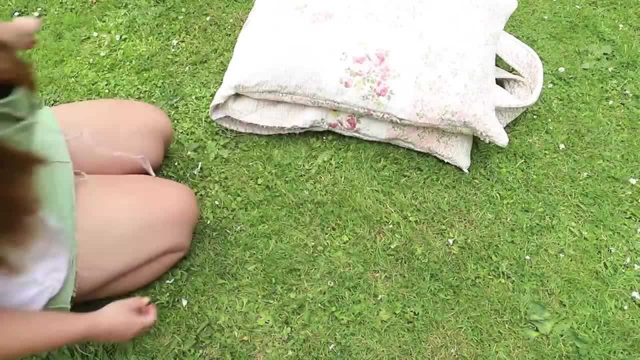 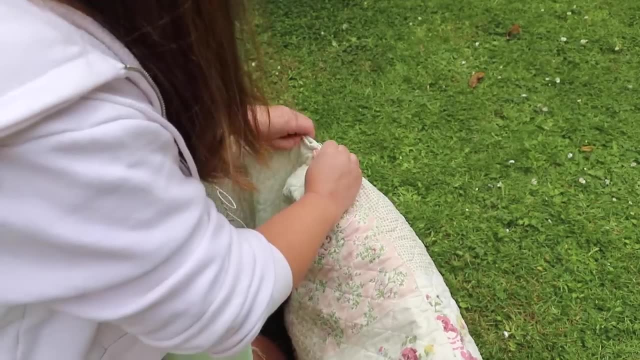 I'm going to leave a gap on the side now so I don't make a crease where I'm going to fold down, and then I'm going to do the same thing. I'm just going to take a bit of seam allowance and tap it at the bottom of the fabric. so 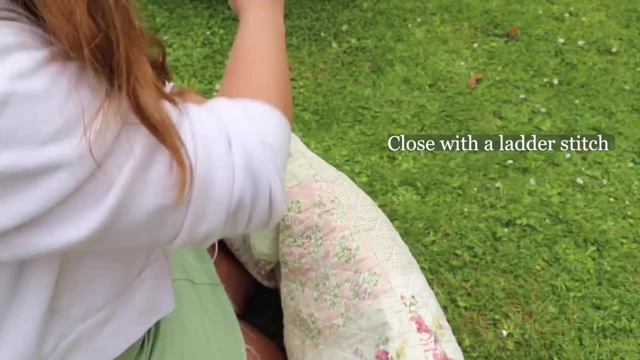 it doesn't flow all the way down And I'm going to leave a little cut on the top of the fabric to give more volume to the top of the fabric. So I'm going to leave a gap here, right here, so I can fold the top part down too. I'm going to leave a small gap here. We were meant to be. You make me anxious. I think I might be stuck on you. I love the things you did. you did for me And for me. it seems that you're dropping clues. There's no need to rush.